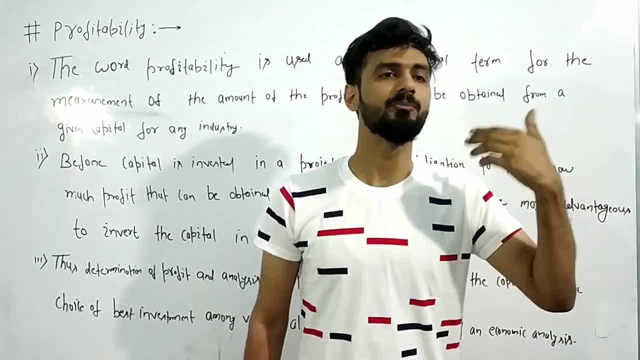 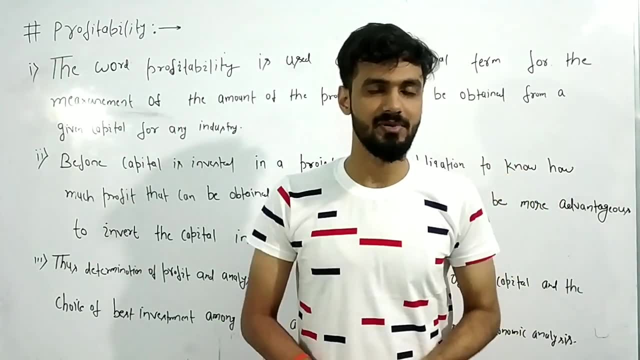 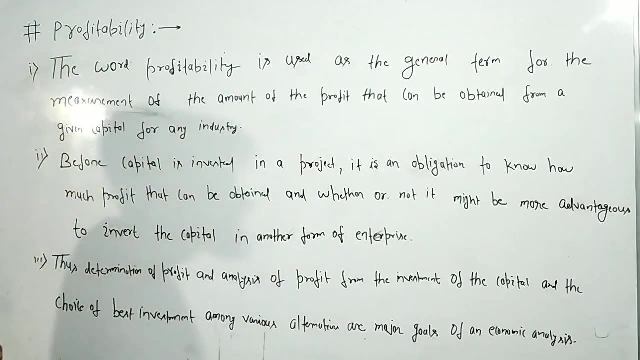 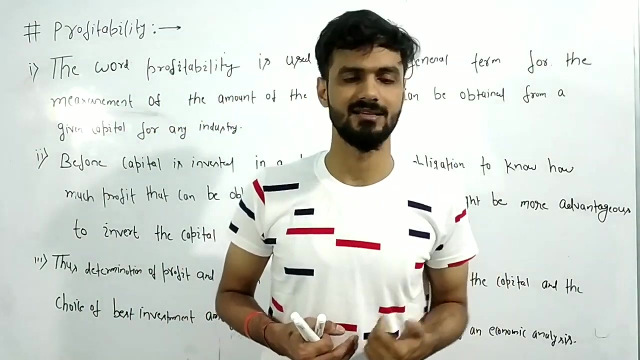 that we have to take in our pocket, and up to which time and in which, at what rate that is going to come from us, come to us? that's major concern in the profitability okay. So, if you will see, the word profitability is used as the general term for the measurement of the amount of the profit that can be obtained from a given investment or for a given capital for any industry. 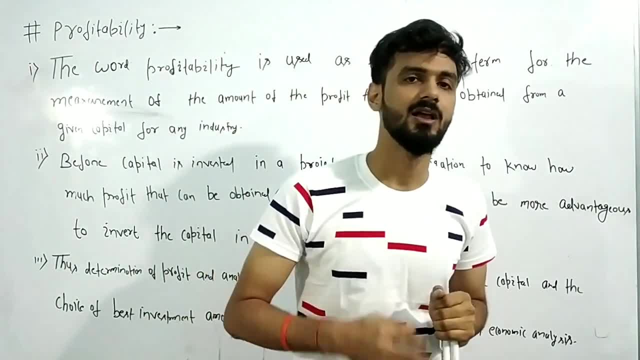 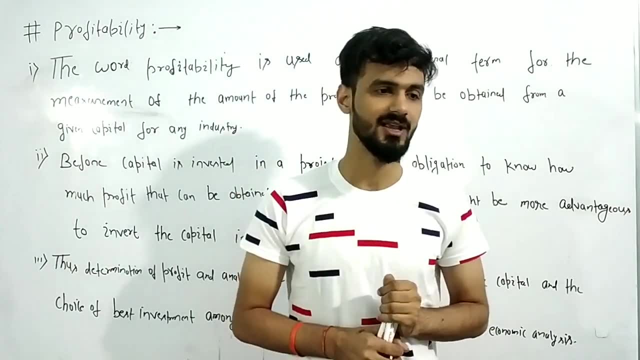 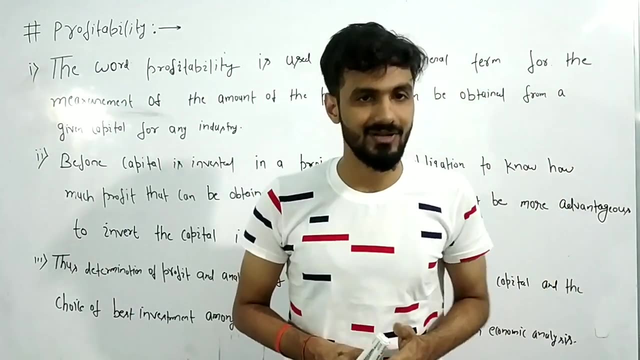 Just understand one thing: if you are going to invest some amount of money- 1 lakhs, 2 lakhs rupees- for any organization or for any industry, okay, That's up to this point, that's okay. It doesn't mean that only you are going to invest money and you want to be, you know, you want to be thinking about your return, okay. 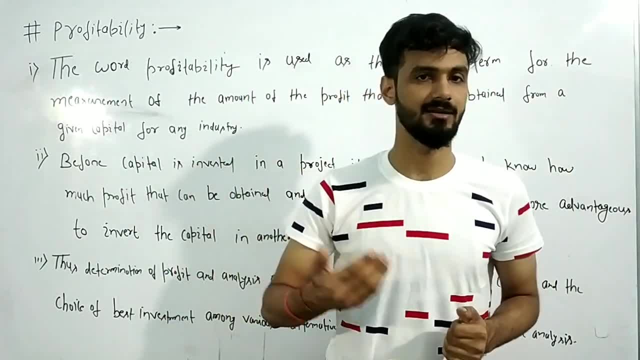 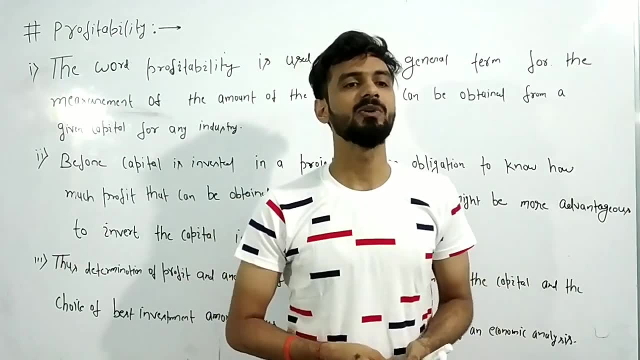 Definitely, whenever you use to invest money on any plan or any project, then definitely there will be something that will be going in your mind that up to what time or up to which rate and how much amount of profit that can be obtained from this investment. okay, That's the major concern. 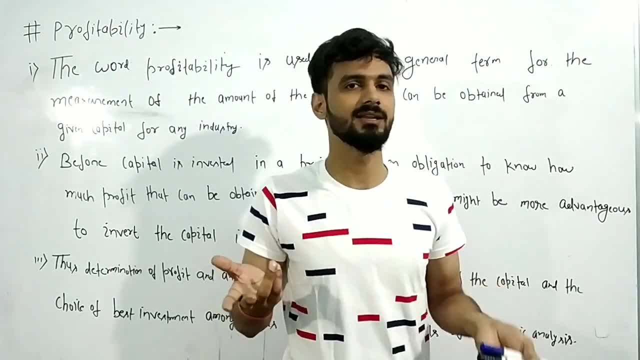 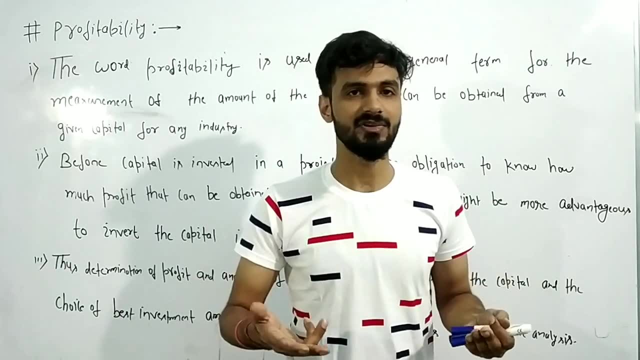 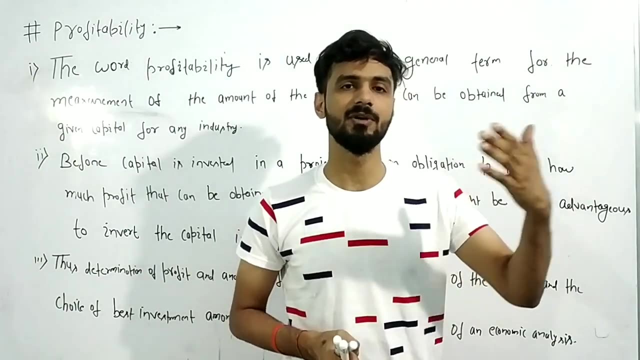 Okay, If you are going to invest any amount or for any capital, for any project, then definitely first thing that you will be thinking about that you will be thinking in your mind that definitely I will get some amount of return from this capital. that's what we use to invest the money, okay. 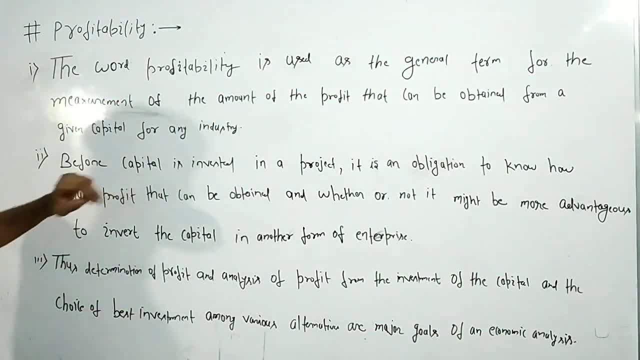 So that was the major concern here. Now, if you will see, before capital is invested in the project, it's an obligation to know how much amount of net profit that can be obtained whenever you are going to invest money on any project. 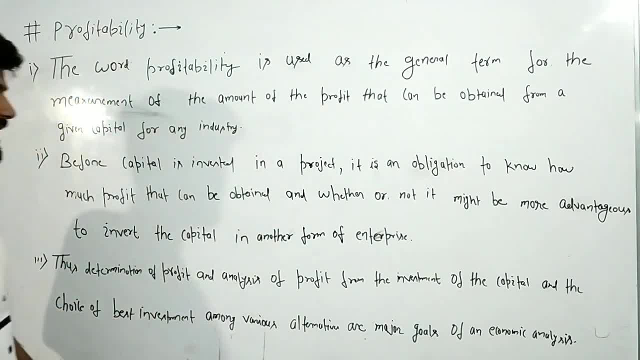 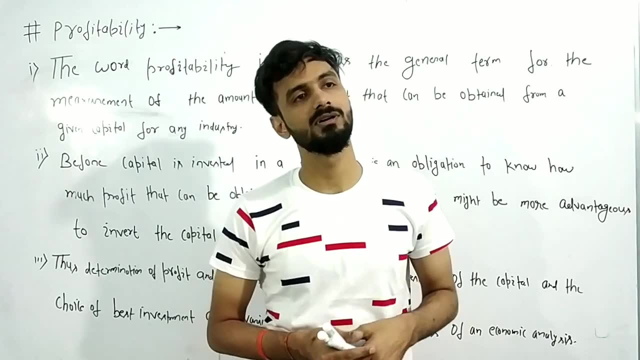 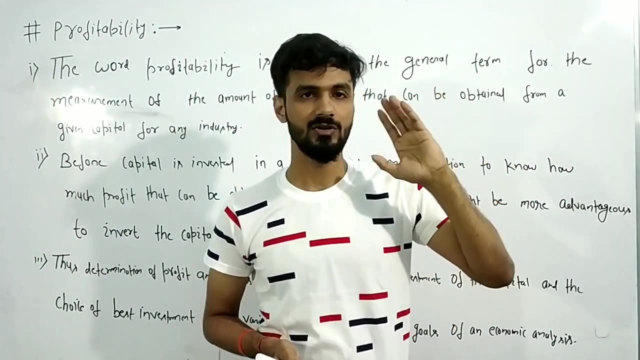 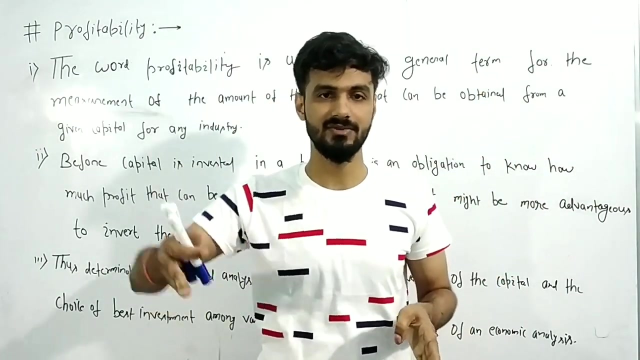 Okay, However, or not, it might be more advantageous to invert the capital in another form of the enterprise. Another simple thing: what needs to happen? if you are going to plan about investment, for any capital you will be, there will be three to four idea that will be running parallel in your mind that if we are going to invest that much amount of capital here, that much amount of capital in some another way, that much amount of capital in some another way, you will be thinking differently that how much money or how much money you are going to invest in that project. 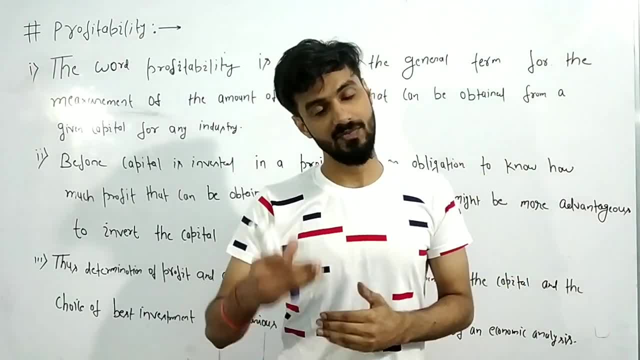 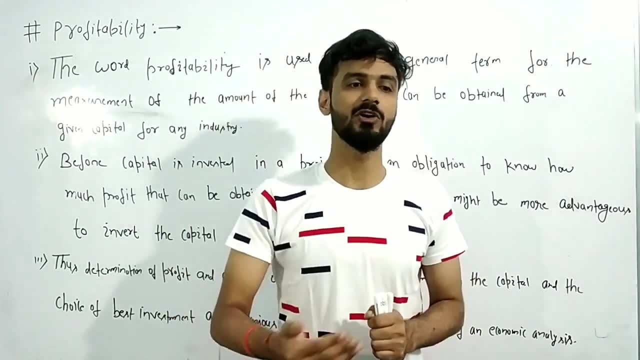 much profit that can be obtained from first project, the same capital you are going to invest there. some people, you will be thinking that, okay, up to what year? up to what year we will get the invested amount, we will get the return of the invested amount. okay, so, 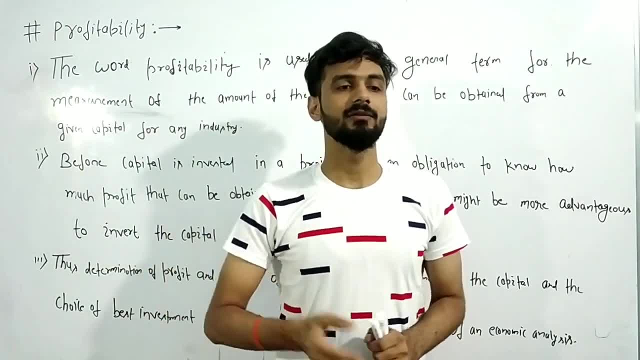 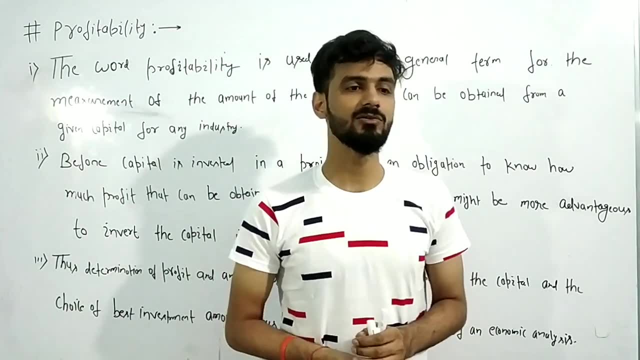 or some people will be thinking, apparently, that we, in which rate we will be getting the return from that capital investment. okay, so there are so many things that will be going in your mind that up to what year, in which rate or how much profit that can be obtained. 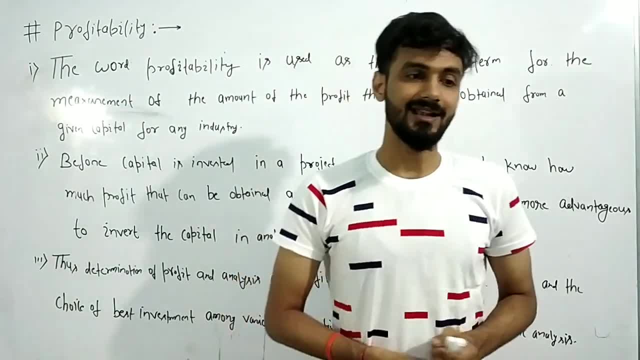 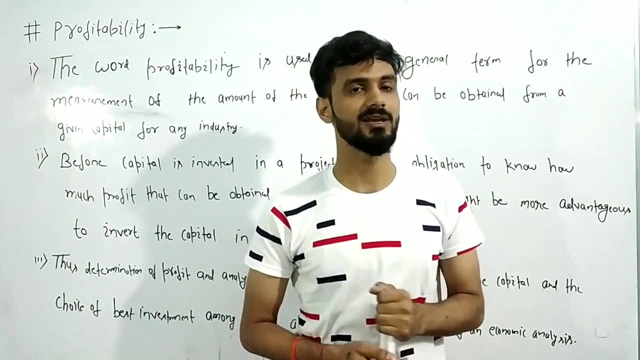 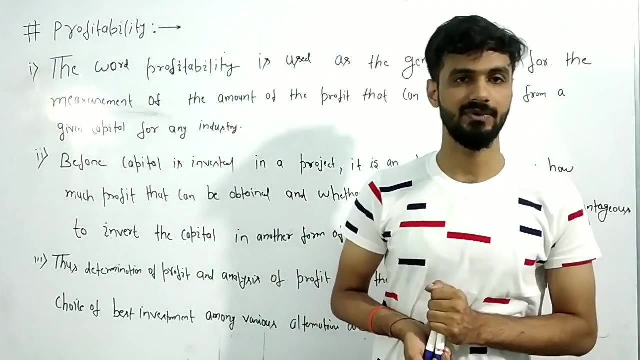 from the given investment. okay. so in that that judgment becomes very intriguing there. okay, because it will be very ambiguous for you, okay, in which way we have to invest the capital and where we have to invest the capital. because if you will think for any investment what you will see from there, if you just understand one thing, you are going to invest 5 lakhs. 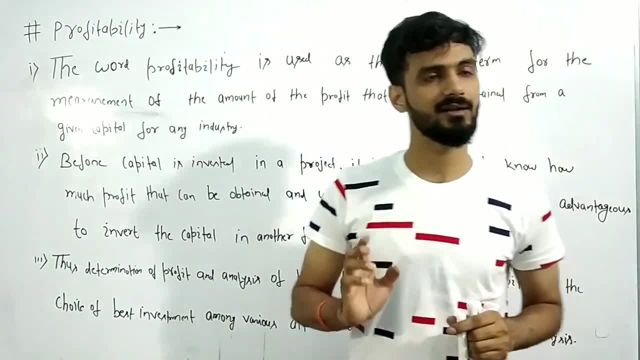 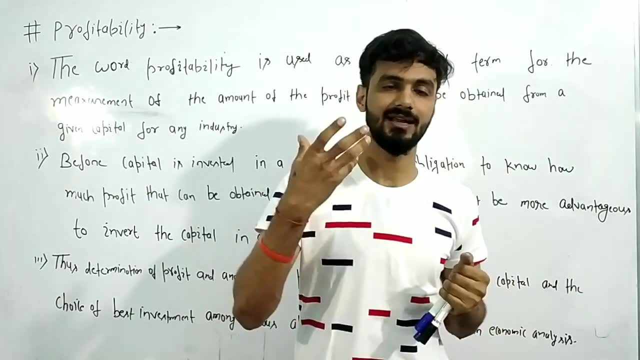 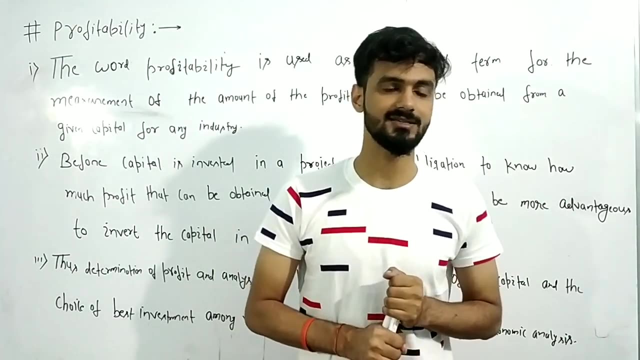 for any plan? okay, 5 lakhs for any project? Okay, understand one thing: and you are thinking the profit, okay. so, because after 5 years you think that some profit we will get or some return we will get from this project, okay, it's okay up to this year, this things, it's okay. now, understand one thing, each and every. 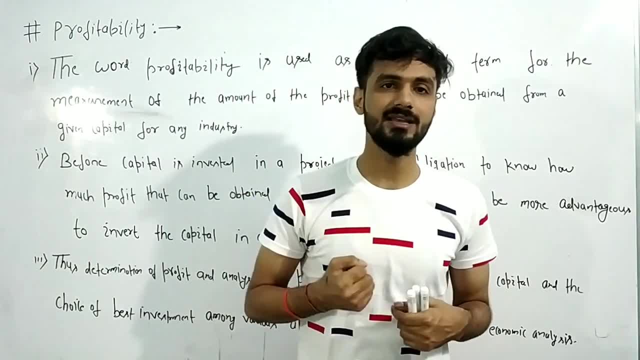 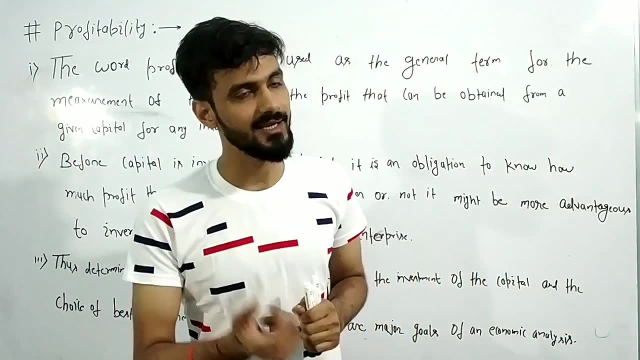 year, just first year, second year, third year, fourth year. the value of money is going to be change each and every year. money, the value of money changes. okay, because already you all know the time value of money. I think okay, and if you don't know, then definitely I will. 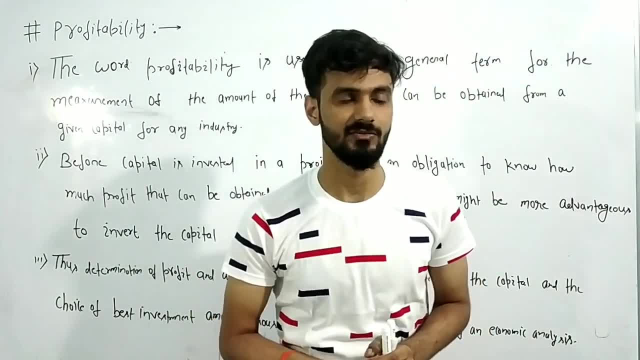 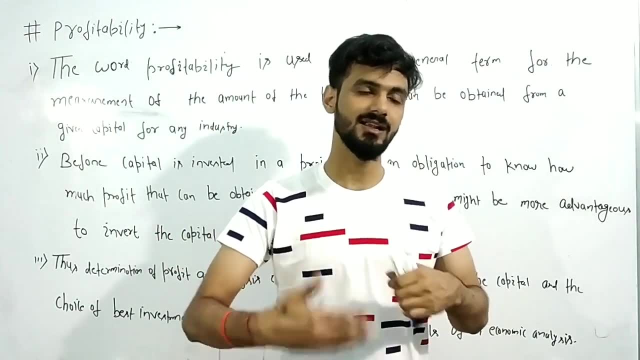 tell you the time value of money In this topic. okay, because we have studied this topic. okay, so each and every year the time value value of money used to change. so each and every year the profit is going to be change. and if the profit is going to be change, definitely that will strike in your 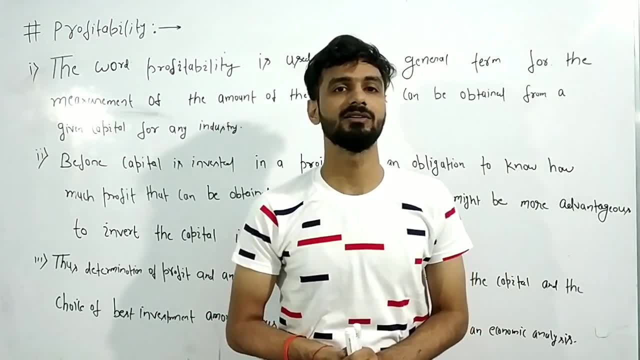 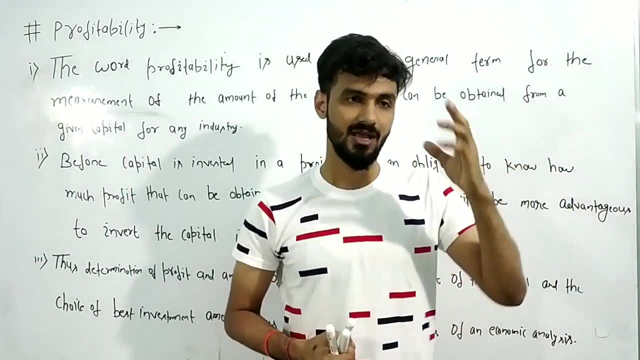 mind that after 5 years, how much amount of profit you are getting? okay, because inflation, deflation, is a natural phenomenon. it has to occur every year. okay, because this is totally related to amount of the value of money. okay, because if the value of money is going to, 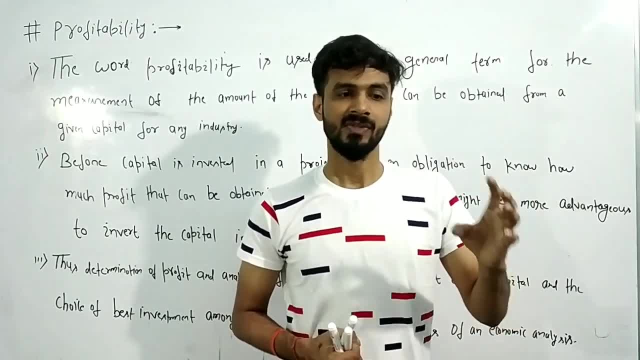 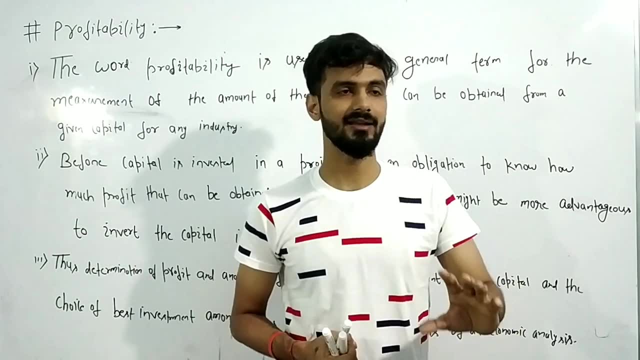 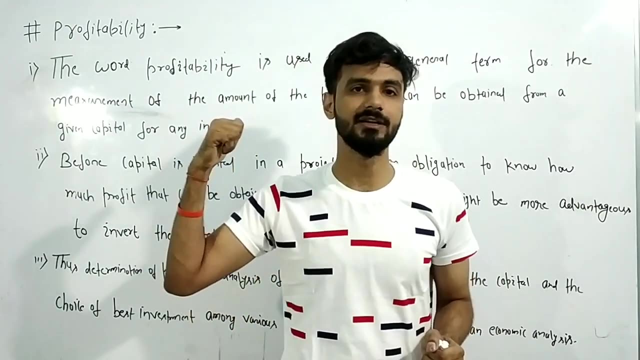 be change, then definitely the profit is going to be change for any project. so you can't only think about profit. okay, only thinking about profit is very difficult thing and in that situation you have to go on the some another parameters and there are various parameters that we have to study in this profitability topic. okay, that's why we used to study the 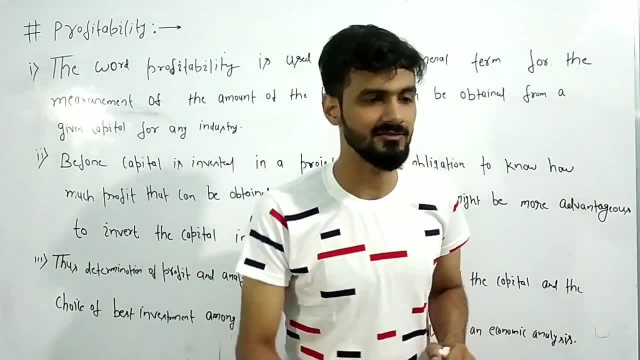 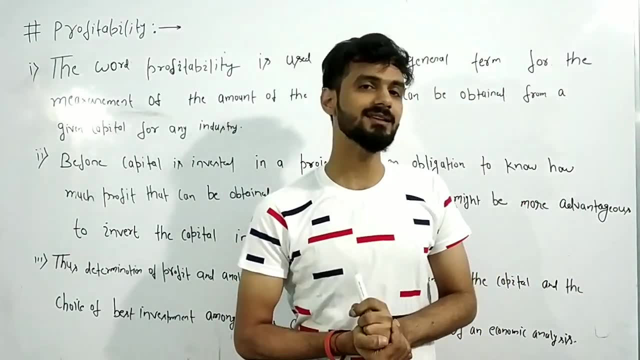 profitability. okay, I think up to this point, you all are clear now. now understand one thing: we have to work on the project as a design engineer because we are a chemical engineer. okay, and as a chemical engineer, we will be working on the project. and due to this particular 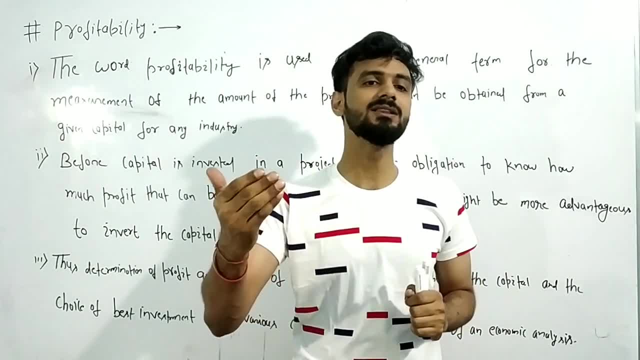 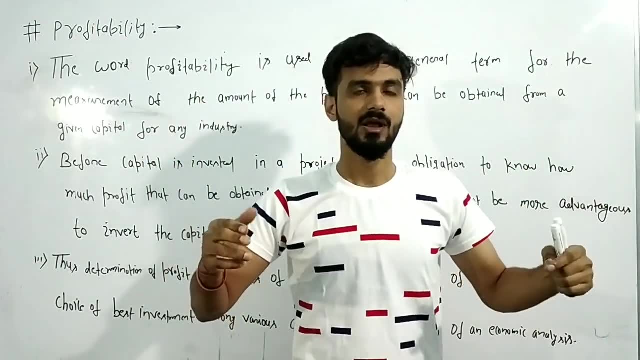 reason, as a design engineer, we have to deal with the capital investment. and if you are dealing with the capital investment, then you have to think whole thing about the amount of capital we are going to invest it and how much money or how much profit we will be getting. 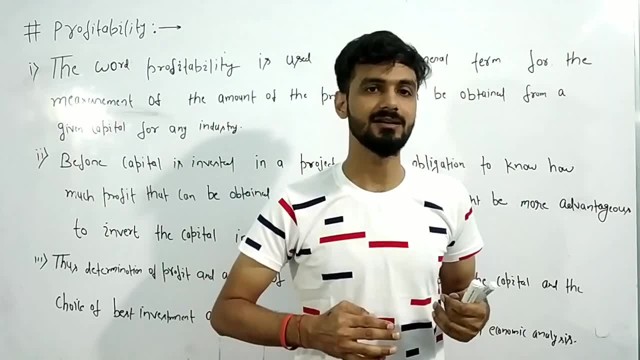 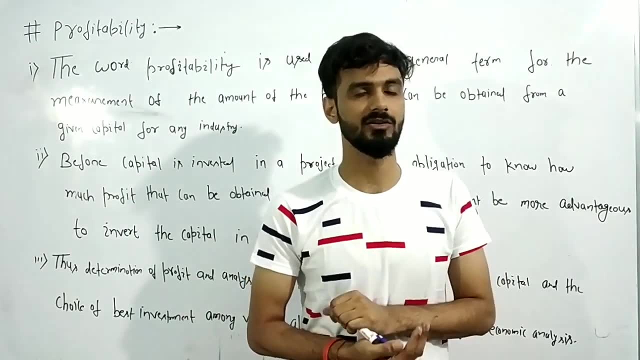 how much time it will take to give us return from that capital investment. okay, these things that you have to build in the while when you are working as a design engineer, okay. so these things will come in your mind. So now understand one thing first. Well, what is a design engineer? 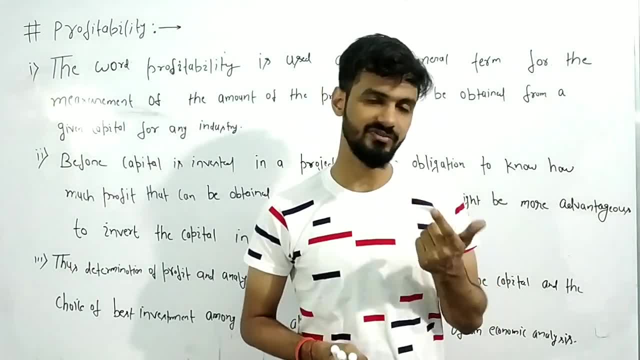 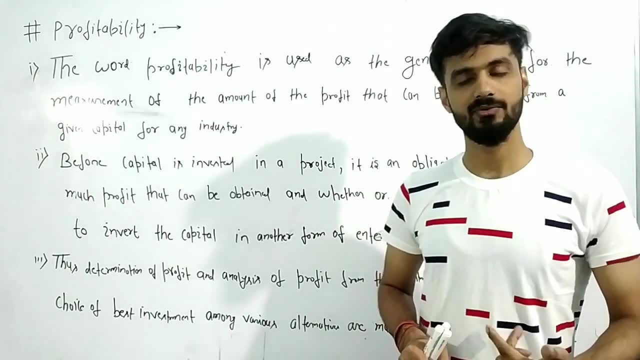 due to deflation or inflation, profit is going to be changed? If profit is going to be changed, then definitely you can't rely on only profit for the investment, Because if you are only thinking about this much amount of profit, I have to get this much amount of profit. 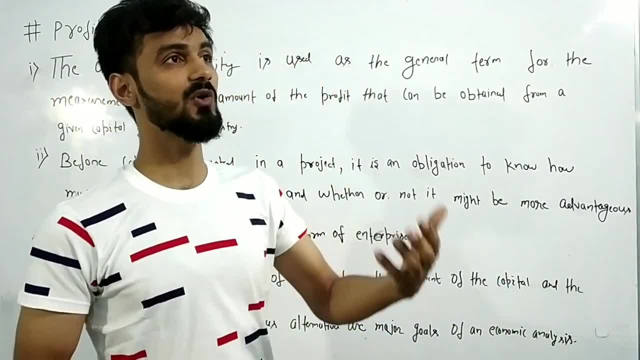 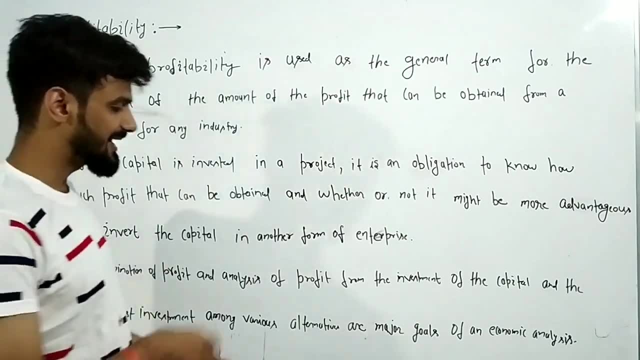 I have to get. So you have to understand up to what year or which rate you will get the profit. That's the major concern here and the solution of this problem that is given by the profitability. My dear friends, if you will think in the profitability we used, 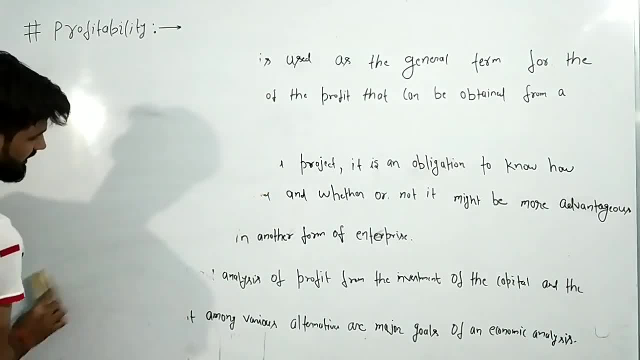 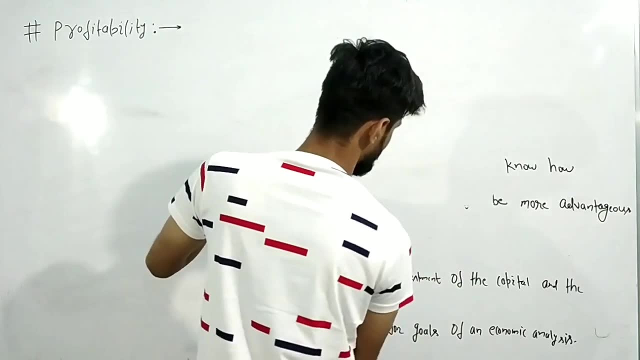 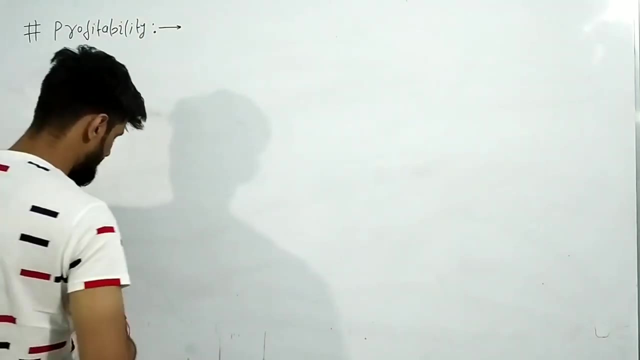 to study about two things, Because this profitability has various parameters and in various parameters we used to study two things: One that used to give the time value of money and that is not reliable on the time value of money. So I am just going to define that term: profitability. 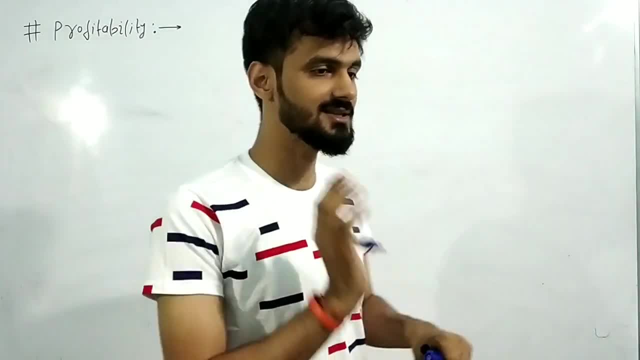 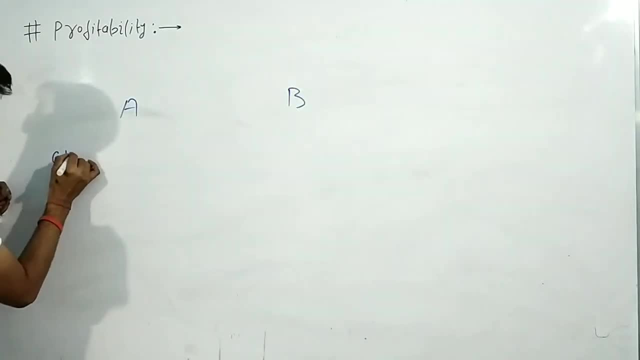 Just understand one thing: I am just selecting two projects. I am just selecting two projects and that project is going to be profitable. So I am just going to define that. project A and project B, A three thing. Now for capital. understand one thing: capital here. 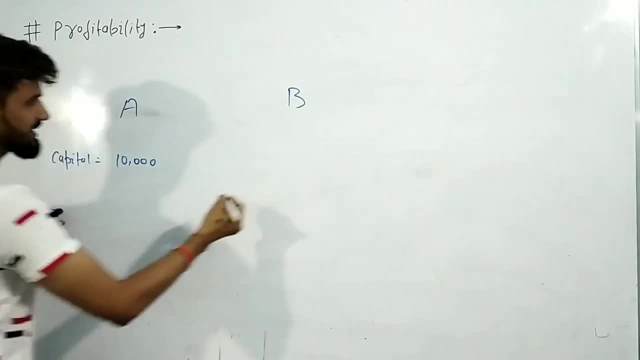 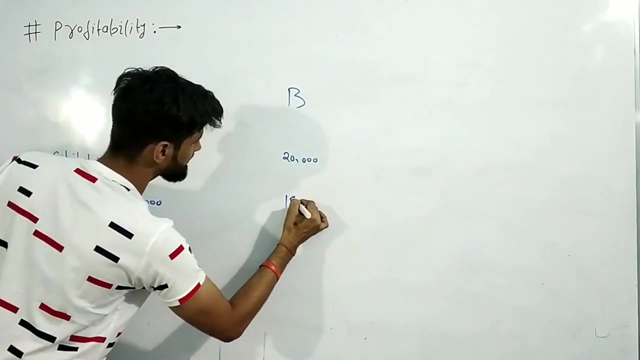 I have invested 10000 rupees on project A and I have invested 20000 rupees on the project B. Now, profit per year, Here profit per year we are getting 10000 and here profit per year we are getting 1500.. These two things you will see. Now understand one thing: what is? 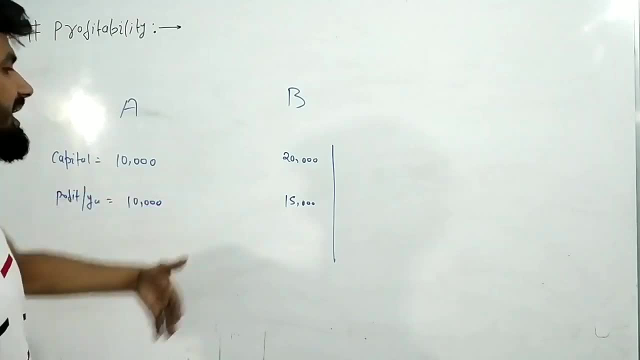 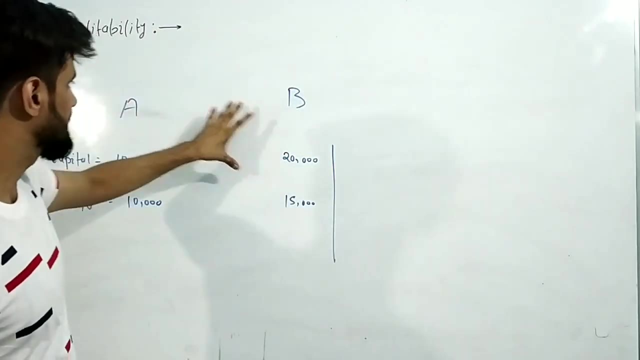 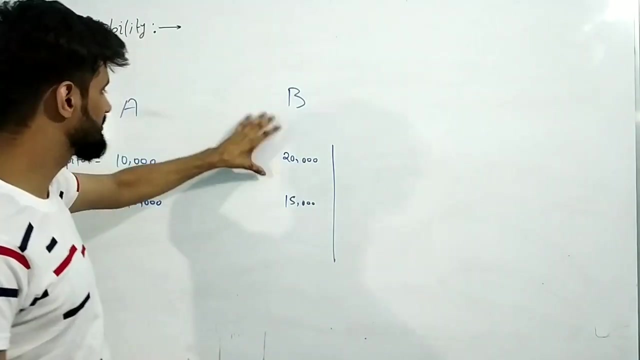 difference in the year between these two projects and in which way we will be thinking about the profitability, How profitability will help us to compare the better investment, which will be the better investment for our project. Because if you are going to invest 10000 rupees and 20000 rupees, then definitely you will be thinking which will be the best. 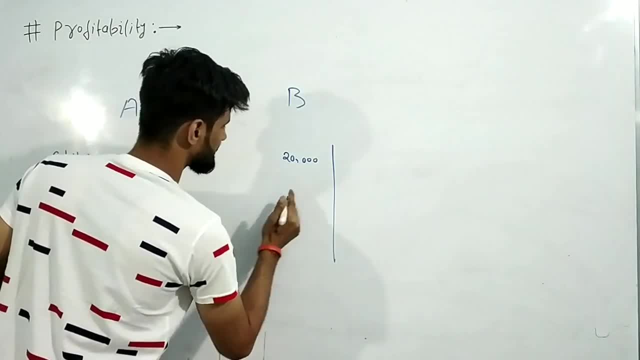 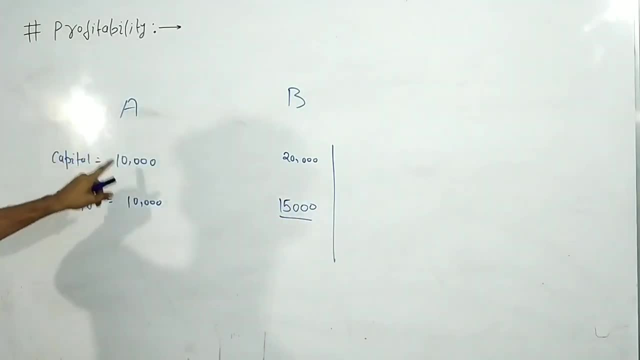 because understand one thing: I am just taking here 50000 rupees. Okay, 50000 rupees means just 15000, it is okay. now Understand one thing: here capital is 10000. here for B capital is 20000.. Here you are getting per year 10000 rupees for profit per year, and here you are. 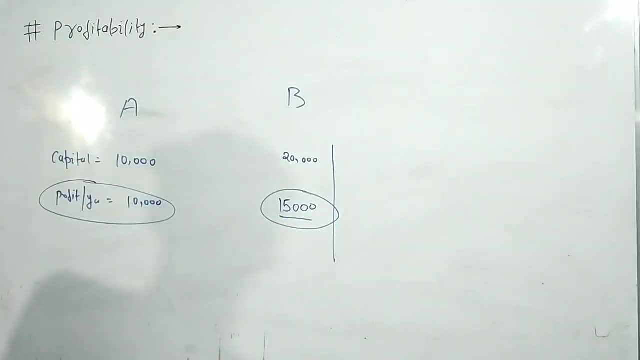 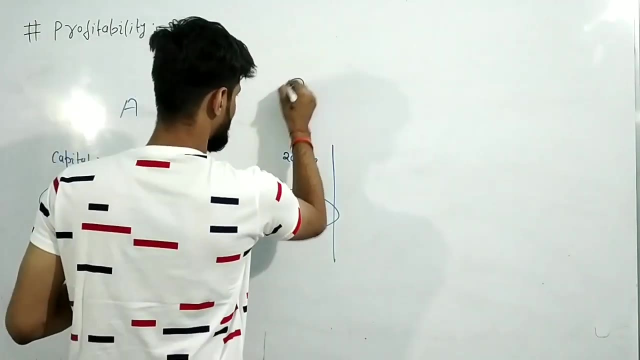 getting 15000 rupees profit per year. Okay, Now understand one thing. So if you will see only profit per year, then definitely project B will be more important. Project B will be more attractive. I think Project B will be more attractive. Why? Because B will be more. 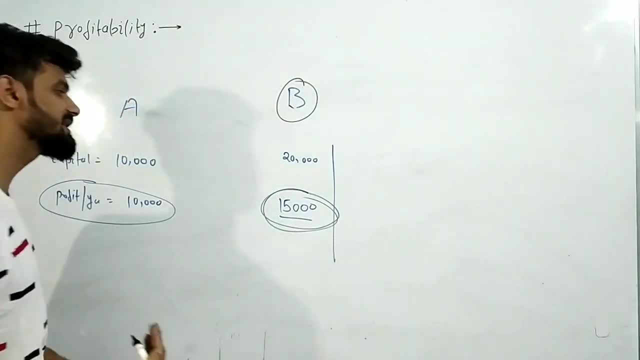 attractive. Why? Because it is giving 15000 rupees per year as a profit. And project A is less attractive. Why? Because it is giving only 15000 rupees every year as a profit. So you will select project B. But understand one thing: you can't see only profit in the 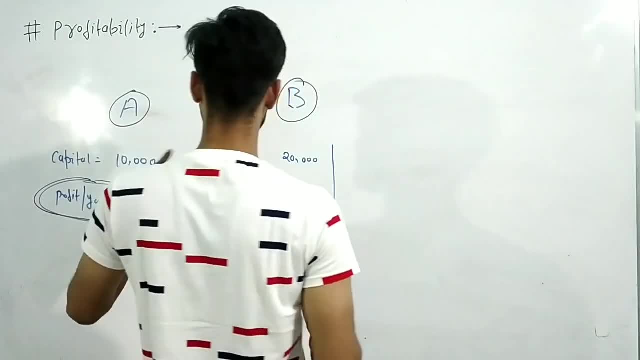 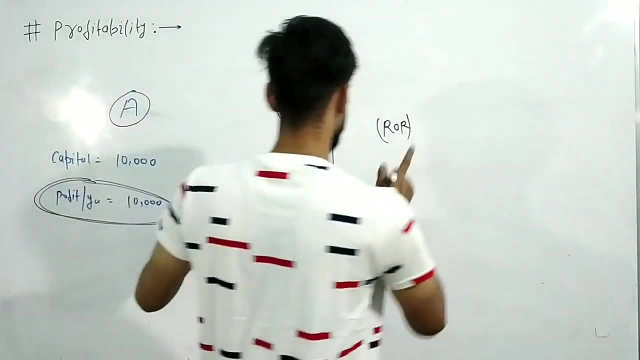 profitability though. Okay. So just understand. if you are going to calculate the rate of return already, I will teach you this topic later on. Just understand. if you are going to calculate rate of return on the project A, That means you are going to calculate rate. 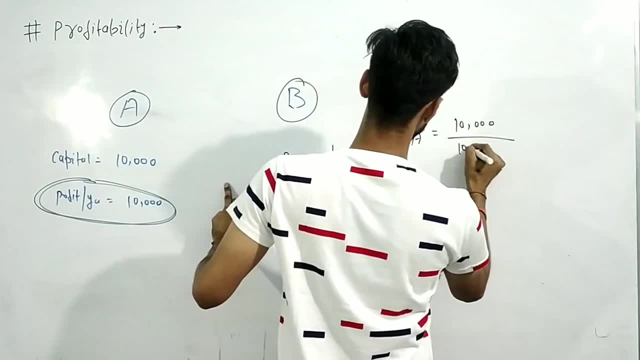 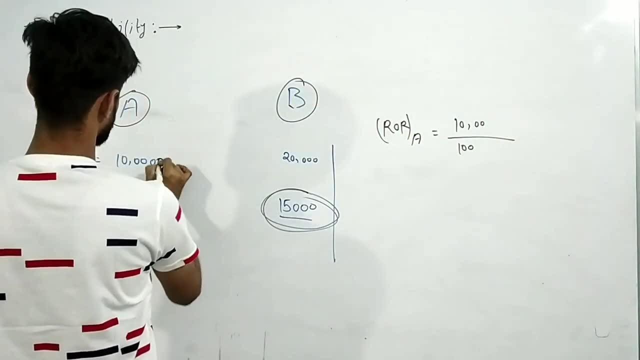 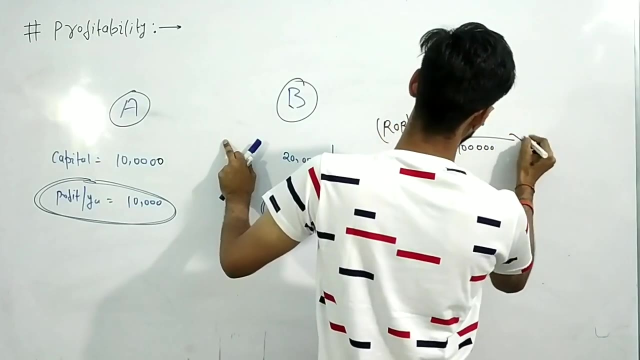 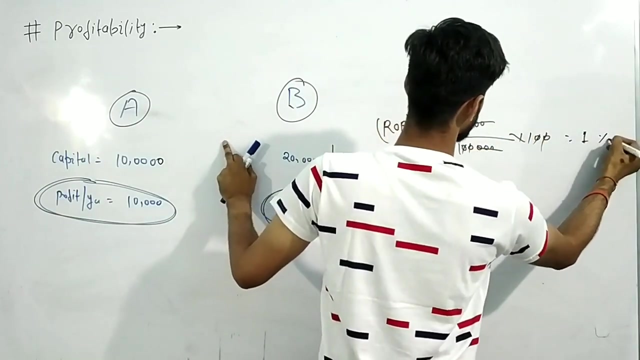 of return on the project B, That will be equals to 10000 upon 10000. just select: this is 1, let's say 2, let's Okay, Into 100.. So now, here you are, getting rate of return as 1 percent. 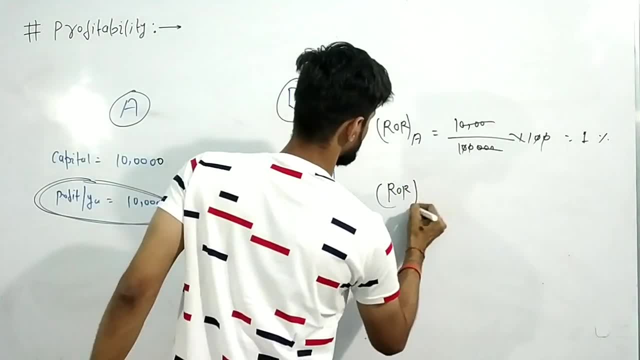 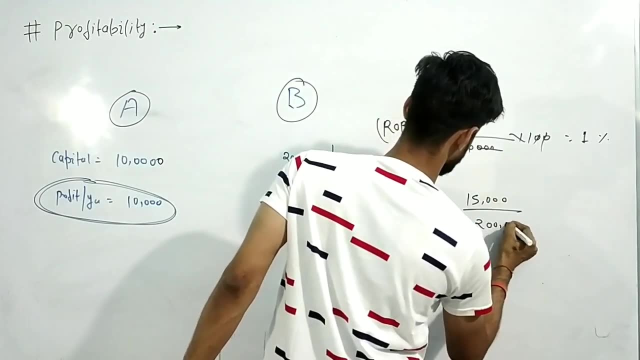 Okay Now here, if you will calculate rate of return for the project B. So here you are getting rate of return as 1 percent. Okay Now here, if you will calculate rate of return for the project B, Then you will get 15000 divided by 2 let's into 100.. So cancel it. 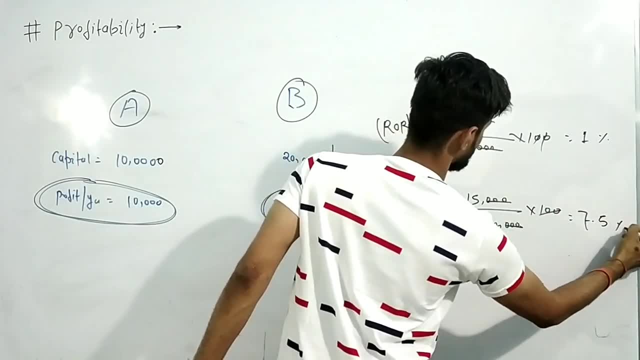 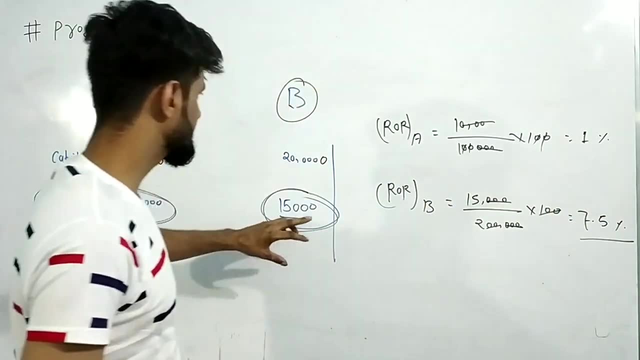 out, Cancel it out. Here you are getting 7.5 percent. You are getting 7.5 percent. So rate of return in project B is 7.5 percent and rate of return in project A is only 1 percent. 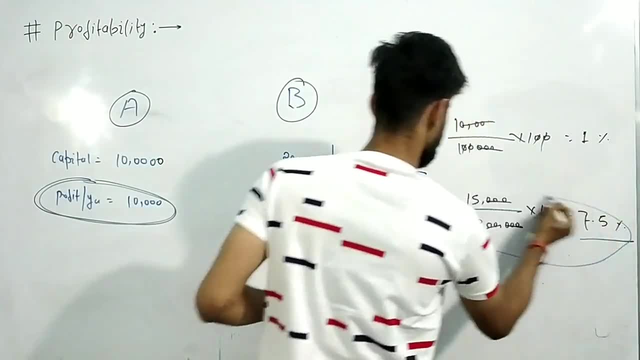 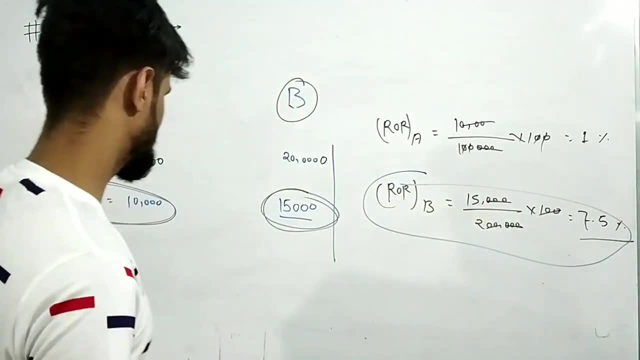 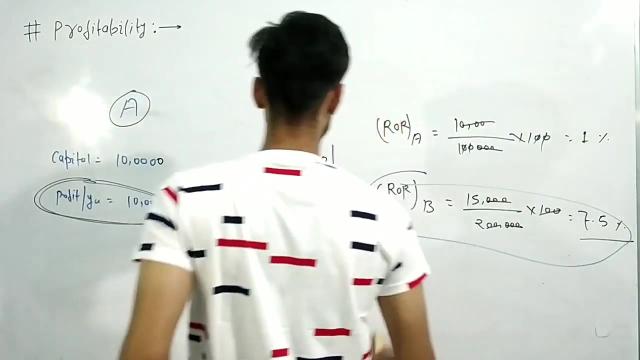 Again, this comes after. project B is more attractive. Okay, Project B is more attractive. Okay, Because here you are getting rate of return is 7.5 and here you are getting rate of return is only 1 percent. So project B is more attractive. Okay, Now understand one thing I am taking 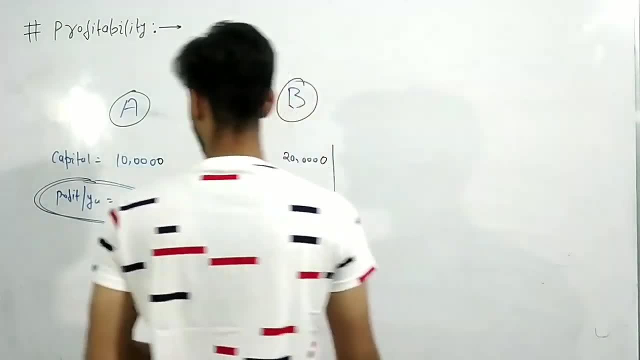 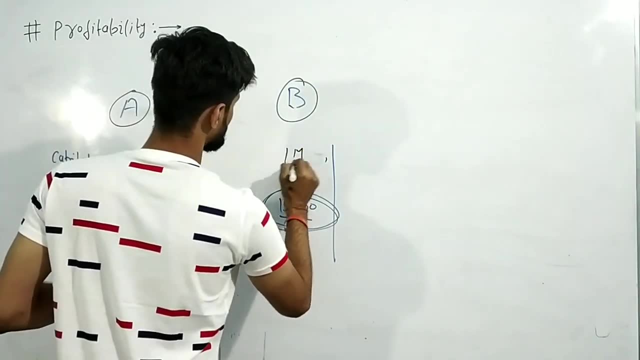 another example. Okay, I am taking another example. Just change the money Here. just understand one thing: Here you just you are going to invest 1 million and you are getting 15000 profit per year. Here you have invested 10000 rupees and you are getting 10000 profit. 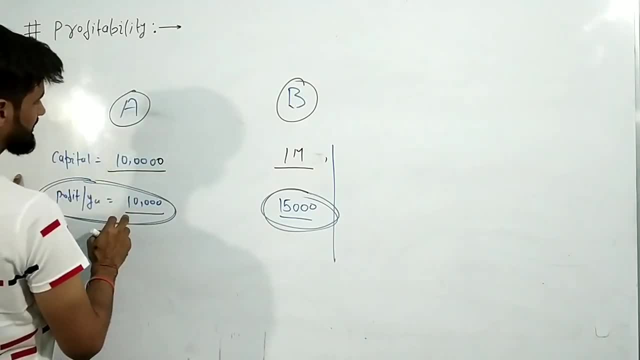 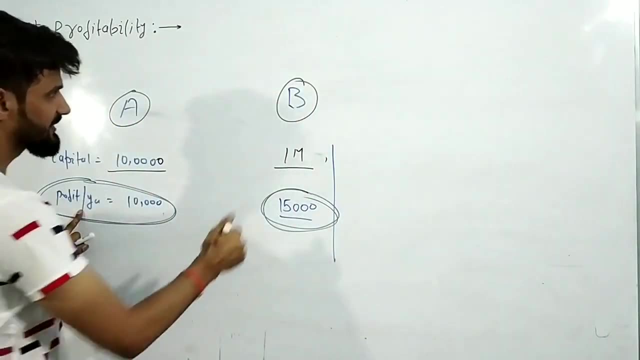 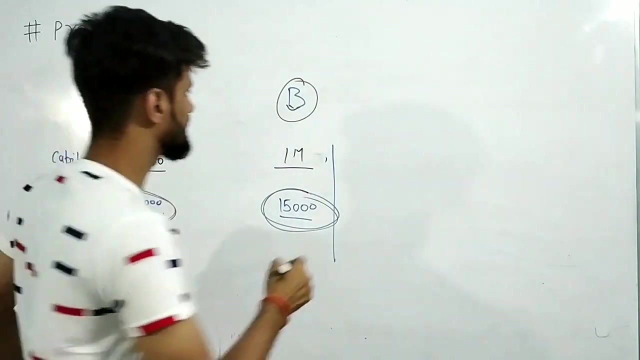 And here you are getting 10000 rupees per month. Now understand one thing: If you will see only profit per year, then definitely project B will be more attractive for you and you will go for the investment for the project B. But if you will see rate of return, then 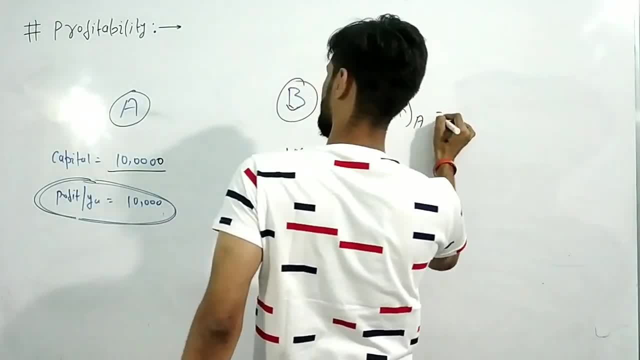 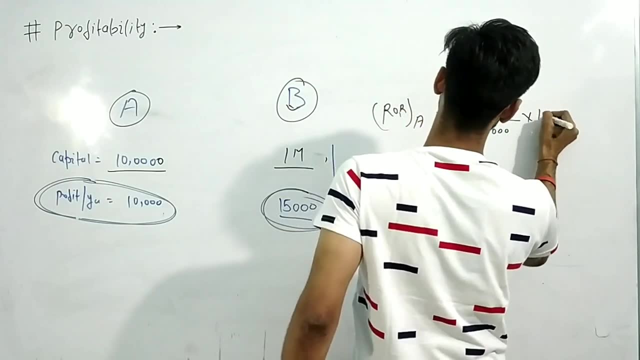 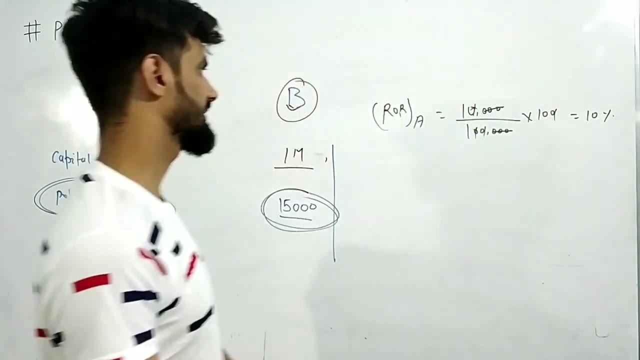 the rate of return parameter says for the project A, that is equals to 10000 divided by 1 lakhs into 100. So if you will cancel it out, then here you are getting 10 percent of rate of return. Okay, And here for project B. if you will see, then here I am just calculating. 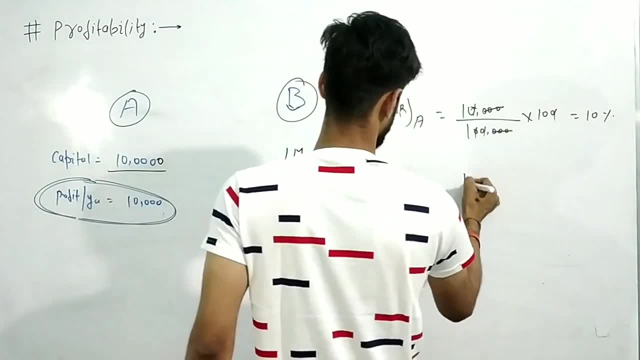 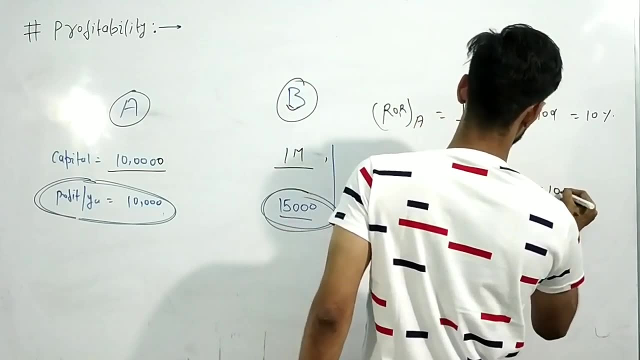 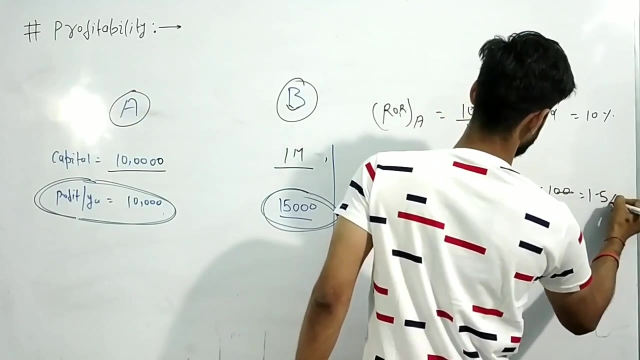 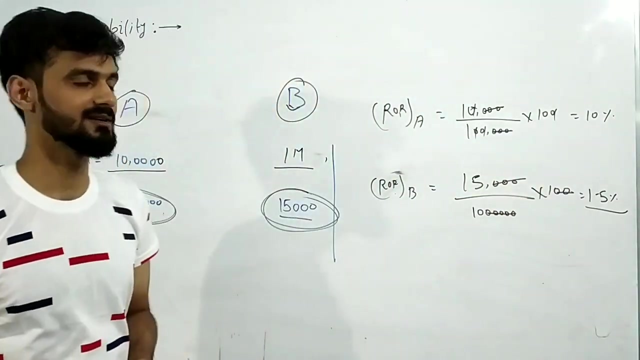 rate of return for project B. that is equals to 15000 divided by 1 lakhs into 100.. Okay, 1.5 percent. My idea is right. Now understand one thing: There are two. Rate of return for A is 10 percent. Rate of return for B is 1.5 percent. Now, if you will consider the rate, 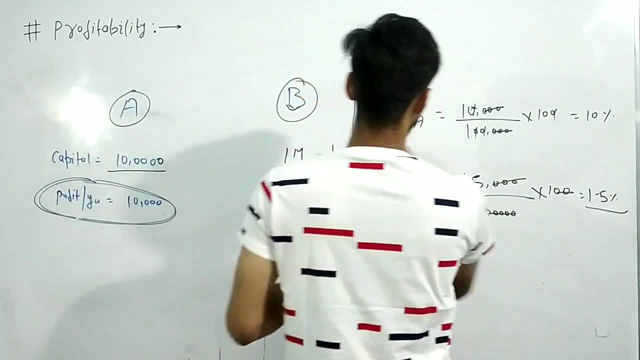 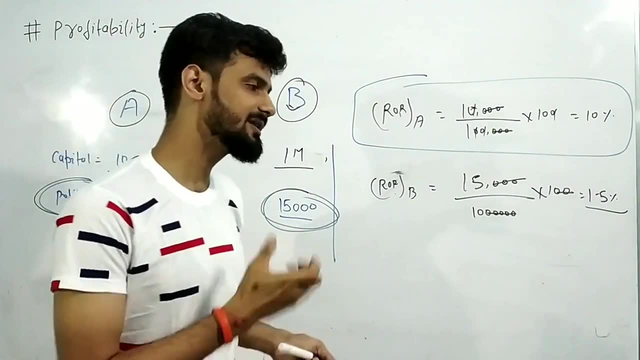 of return parameter, then project A will be more attractive here. So if you will analyze the investment, then there are various things. If you are only thinking about profit, then project A will, project B will be more important, Project will be. B will be more attractive. 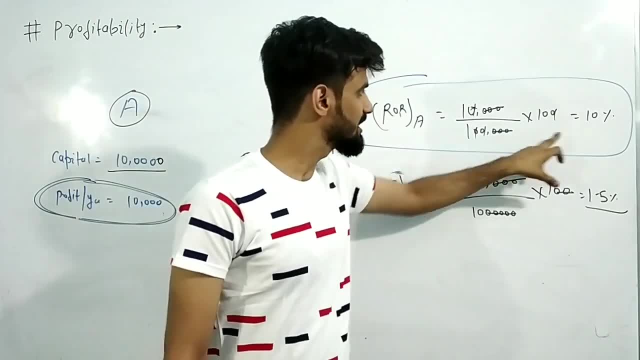 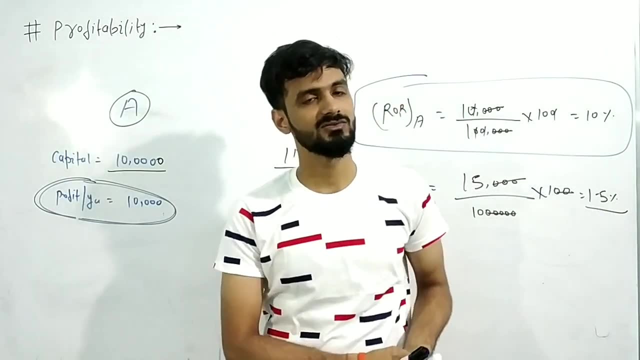 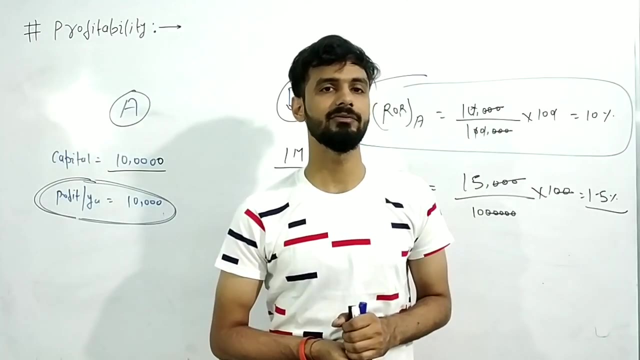 But if you are thinking about rate of return, then project B will be more attractive. So this creates ambiguity in your mind that which is the best parameter. Okay, So this from the analysis of this data, you. I think it is very clear now for you, all of you, that only. 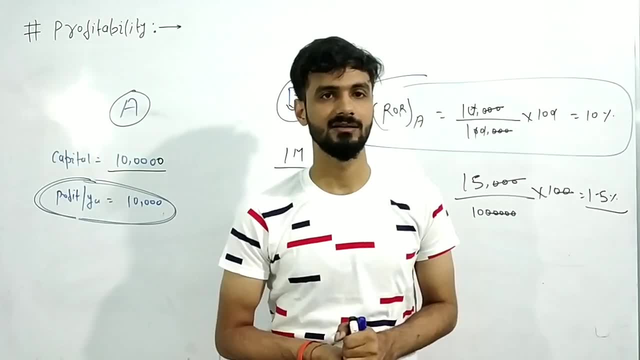 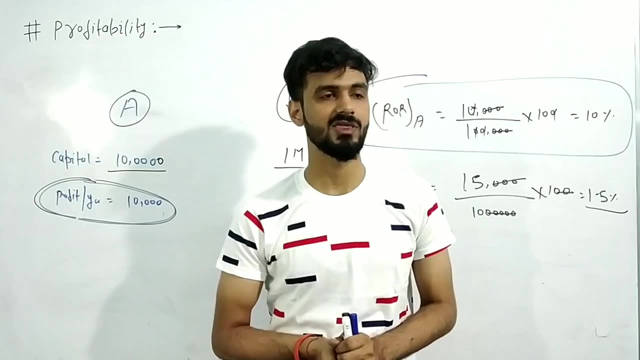 you can rely on the profit. There are various parameters for a project that is going to discriminate whether we, the project, which project is more attractive, which project is less attractive. So just do not rely on only profit. Okay, Now I am going to tell you. 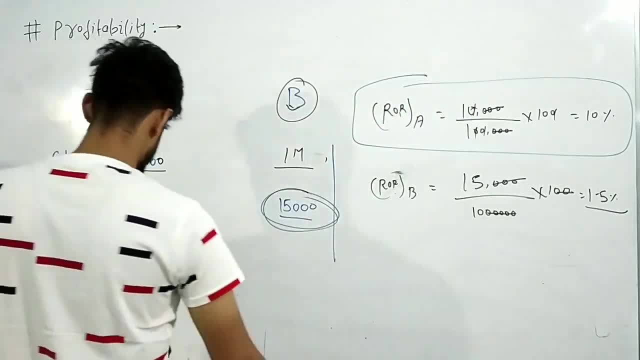 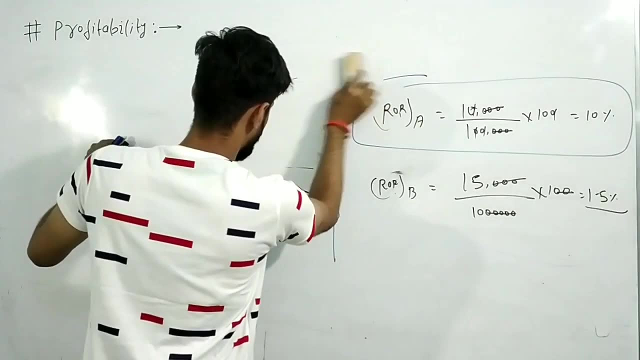 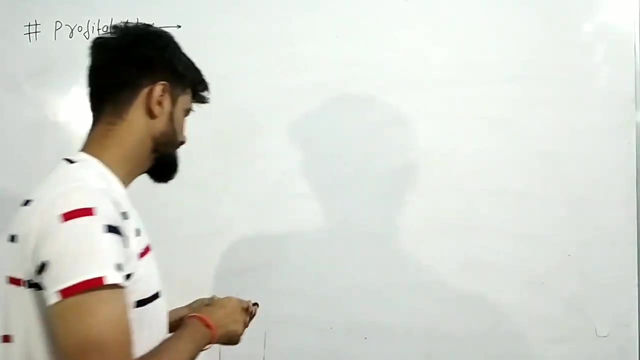 the topics which I have to, which we have to study in the profitability generally, primarily two types of method that we have to study in the profitability Okay, How there are different, different method, and that we have to study Generally. we have to study two types. 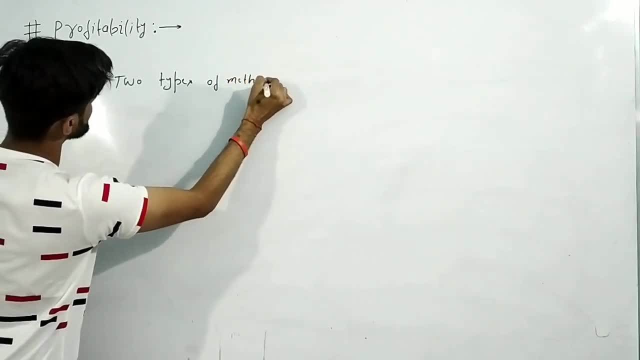 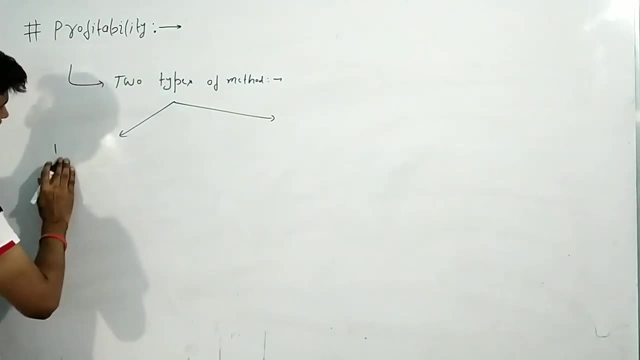 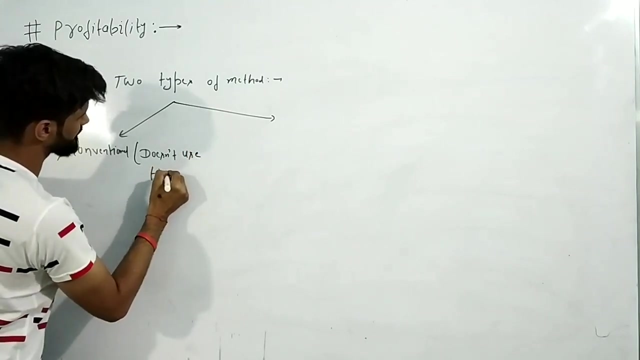 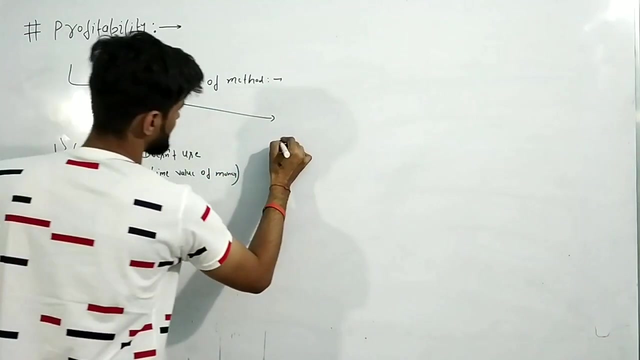 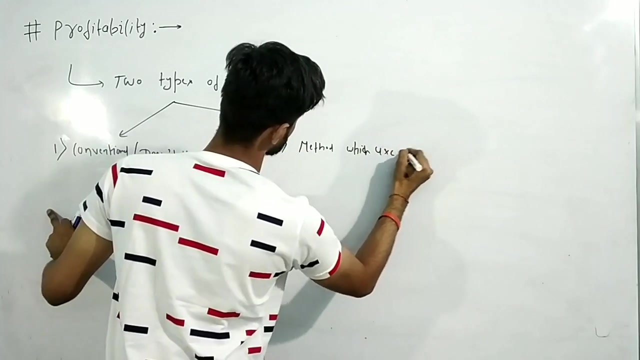 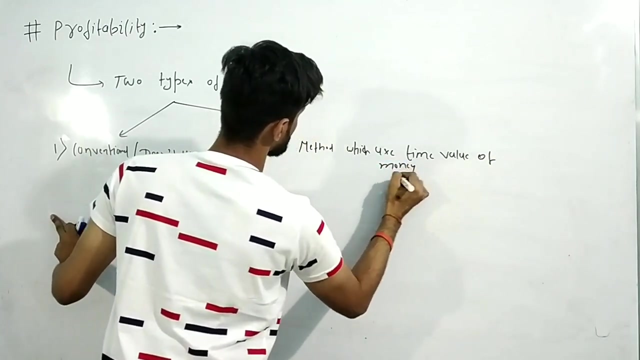 of method. Okay, First method. First method. that is, you can say it is a conventional method. Conventional that does not use time value of money. That does not use time value of money First. Second method, which use time value of money. They are two different methods. 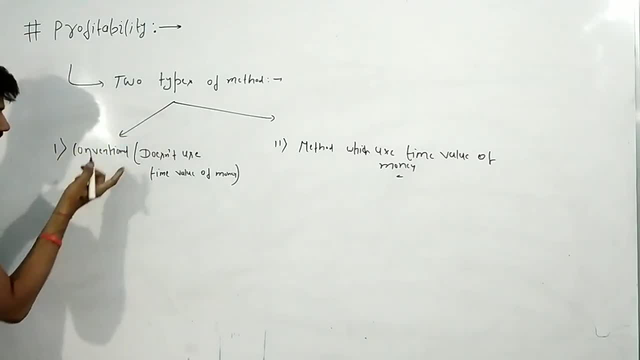 Understood one thing In conventional method: which method, how many method we have to study because there are different types of. if I will tell you this method, which types of parameter that relates to this method, Why we are using this conventional method, Why we are using. 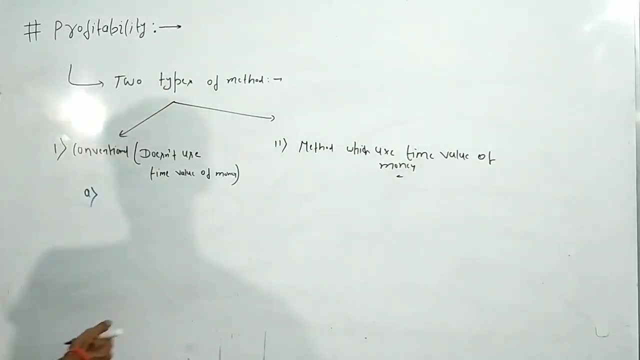 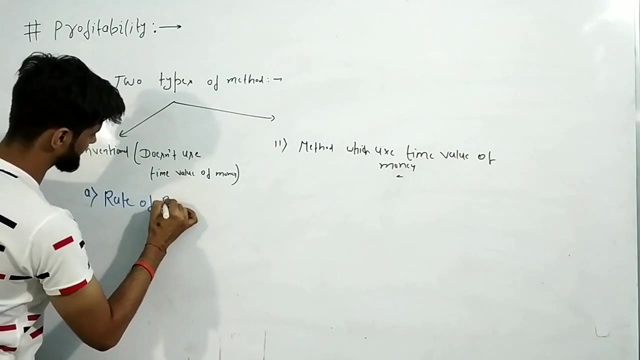 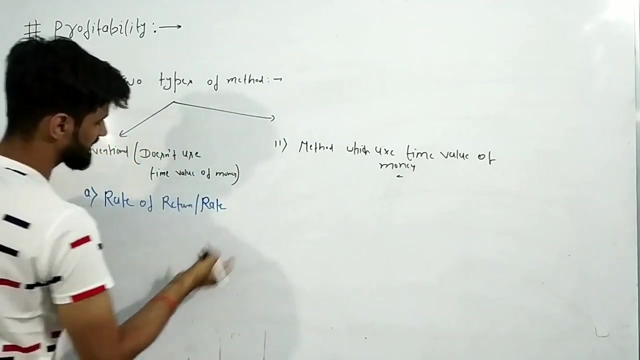 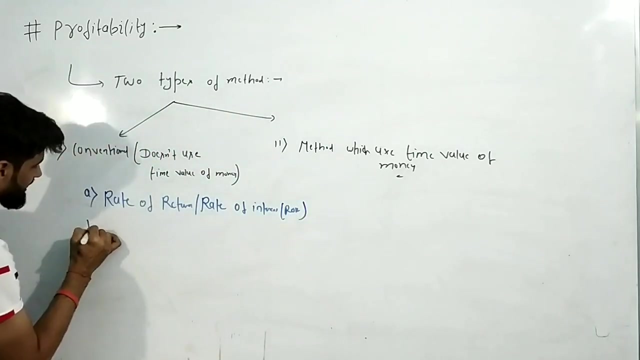 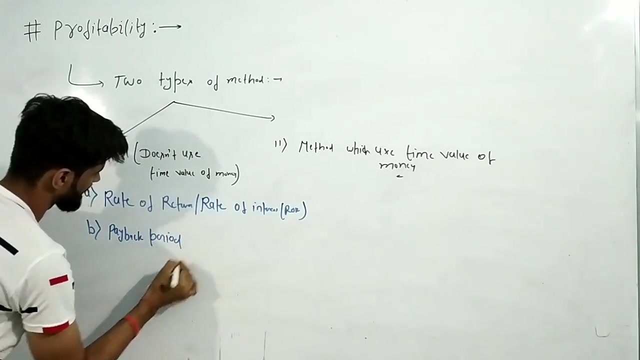 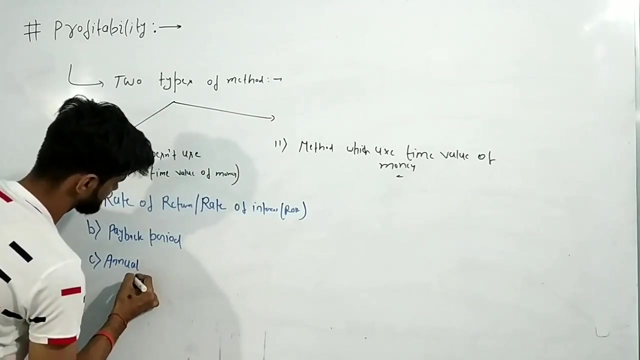 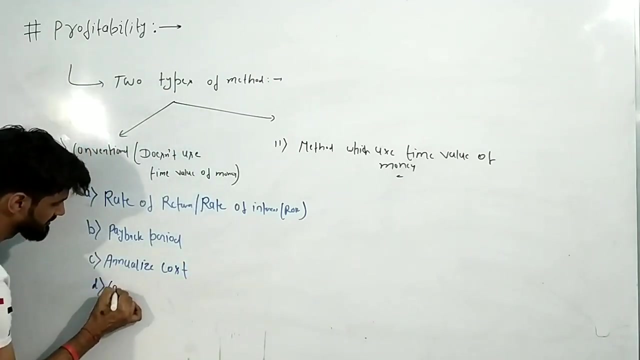 this method. That depends on the scenario I am just writing here. First reason: Rate of return- Okay, Or somewhere else it can be written as a rate of interest, ROR. Second method: Payback period. Third is analyze cost One to one, is capitalize cost, Okay. So 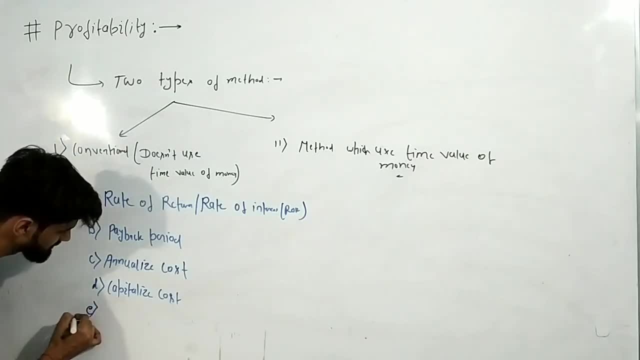 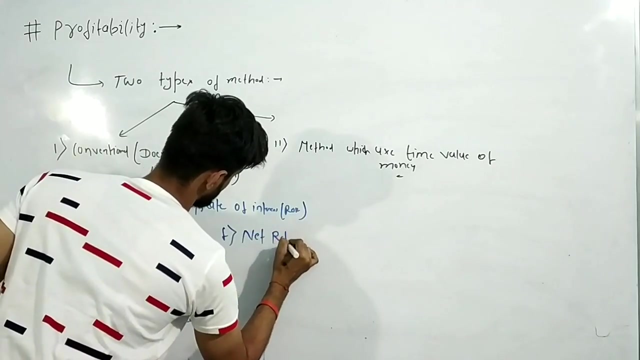 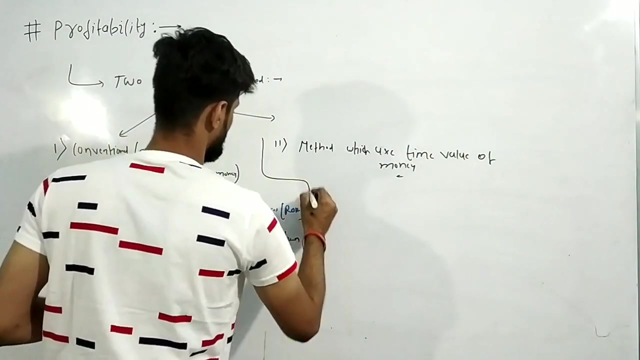 Fifth, one Average rate. Average rate of return, And if you will see F, then that is net return. We don't try to study each and every method. Just I am writing here which which is very important for the eight point of view. I will tell you later, But these are the method that we have to study. 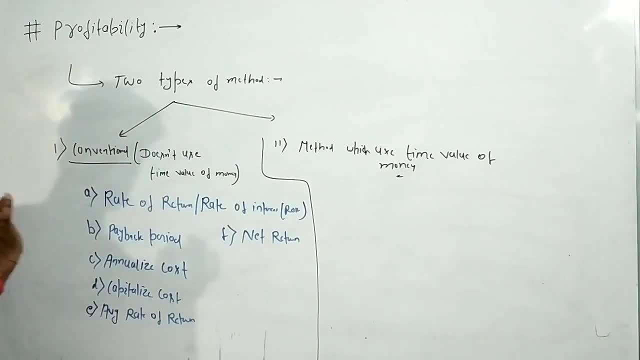 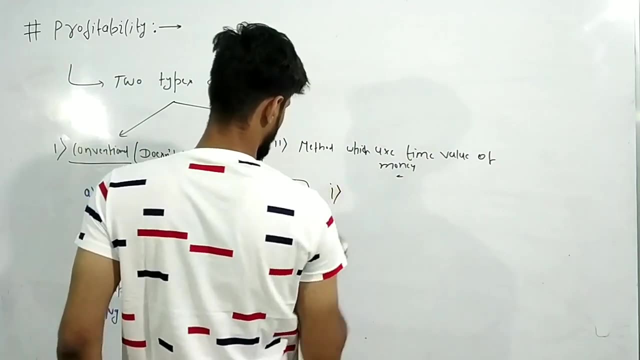 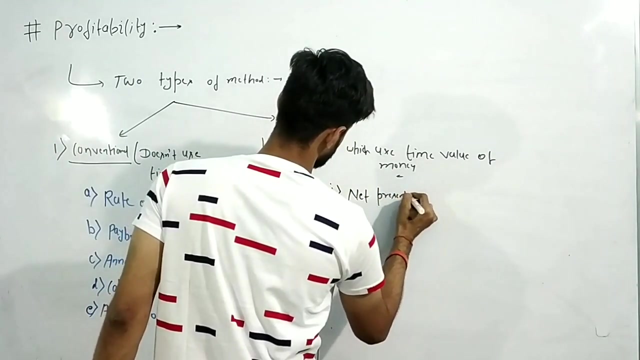 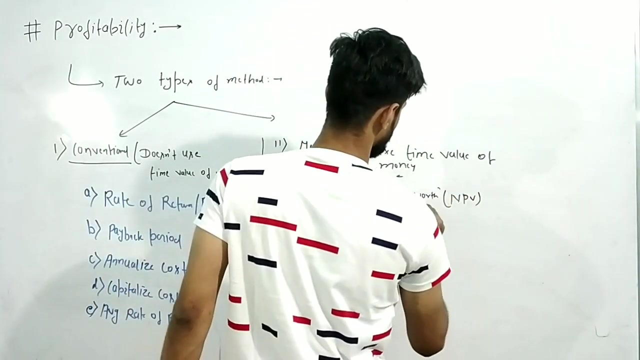 in the conventional method that does not consider time value of money. Now I am going to tell you the second method Which consider time value of money, and first one that comes that lies in this era, that is, net present worth Or net present value. Somewhere else you can see it as a value. Okay, 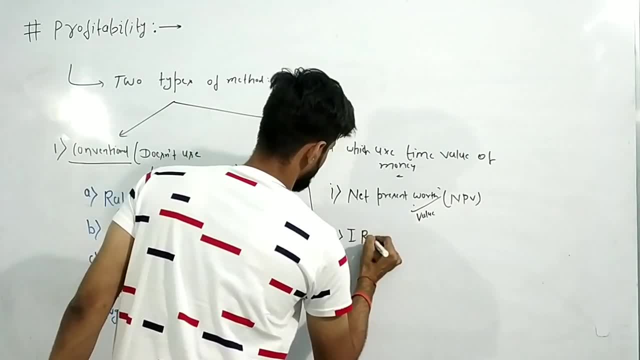 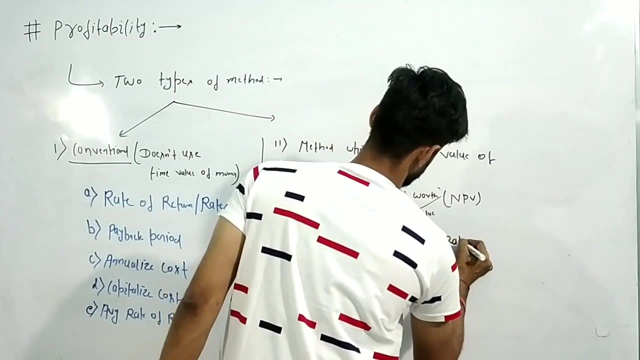 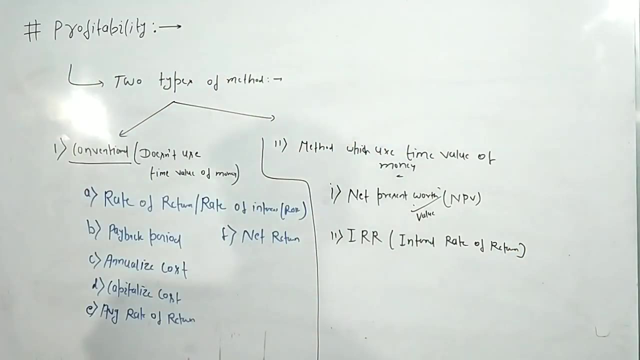 Then NPV. Second, IRR: Internal rate of return. Internal rate of return. Okay, So these are the thing that we have to study in this topic. Okay, Now, now the the thing if you will think about here, then the popularity of this method. 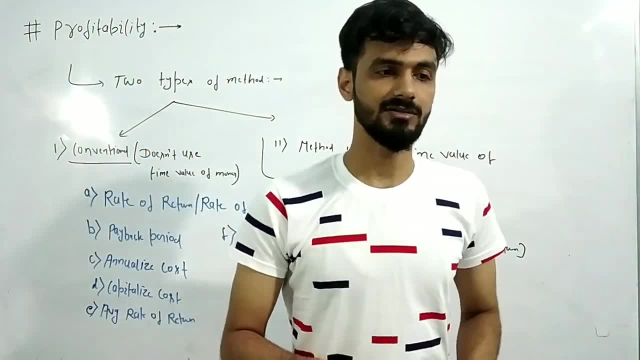 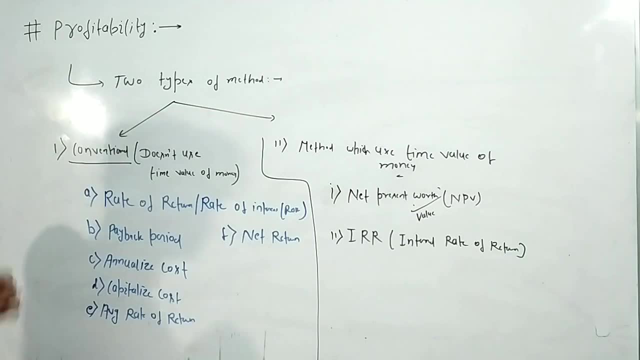 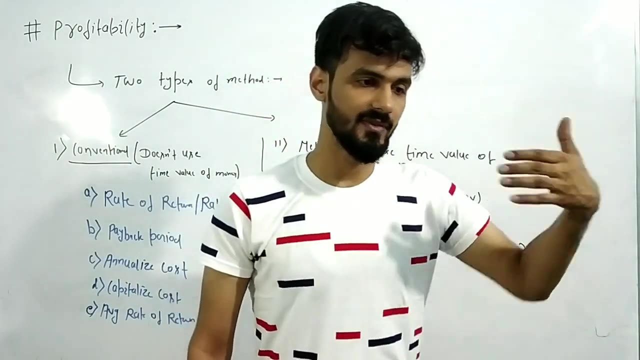 depends upon the size of company. Okay, Because it is very difficult to judge which method we have to use. So the economics has given us the idea that the popularity of this method is gonna be depend on the size of industry. There are various types of industry, if you will see. 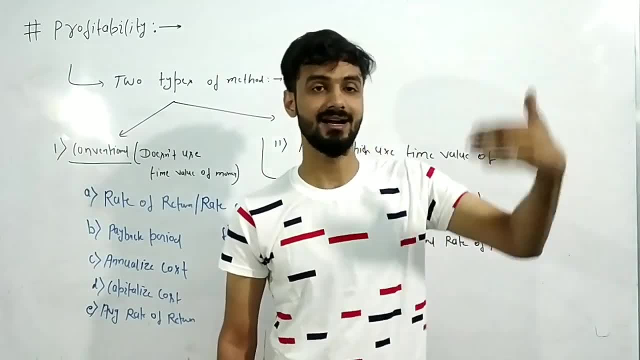 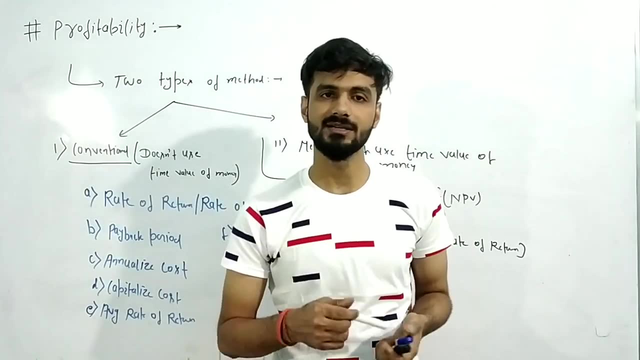 a small industry, medium size industry, large scale industry. Okay, That depends upon situation, that depends upon the various parameters in which way we have to, you know, categorize the different, different types of industry. But here we are going to study the profitability. 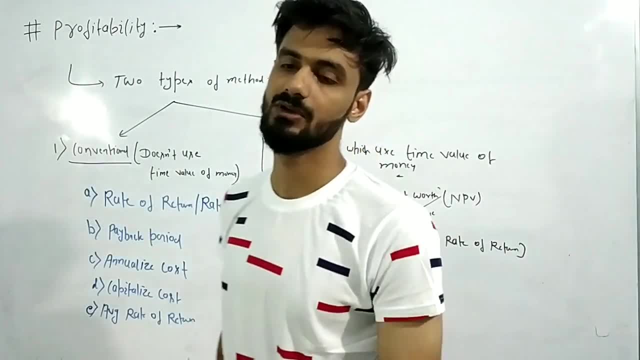 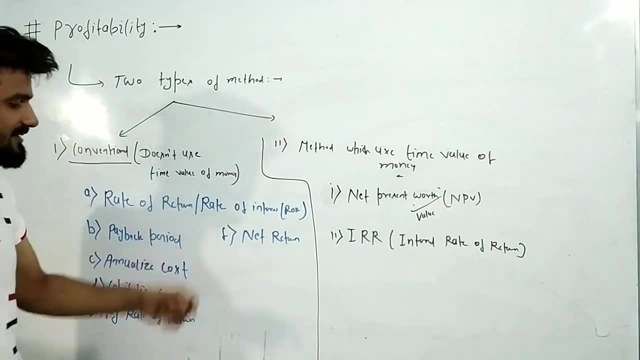 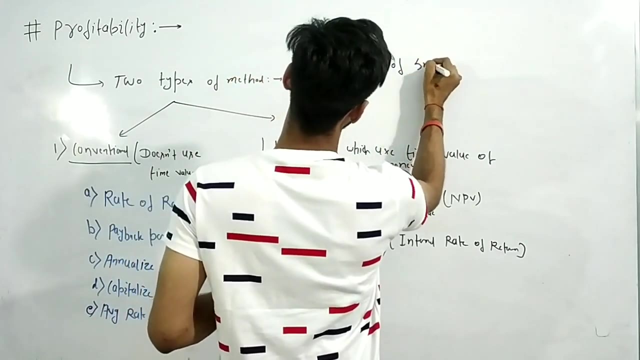 And here we are dealing with the different, different method of the profitability, So where we use the different method. So that depends upon the size of the industry. Okay, Just like conversation, I am giving you a small example, If you will think, 10% of a small industry. 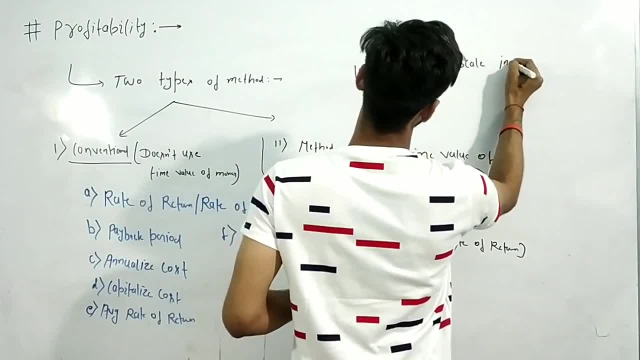 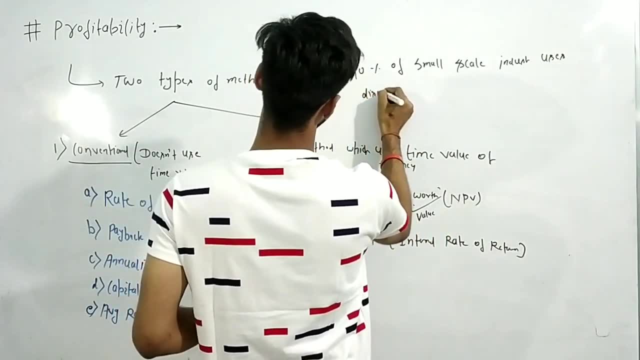 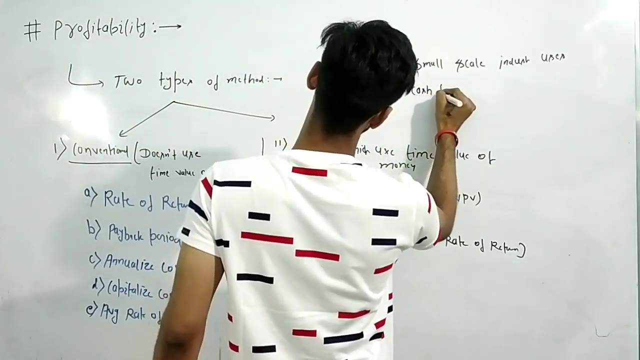 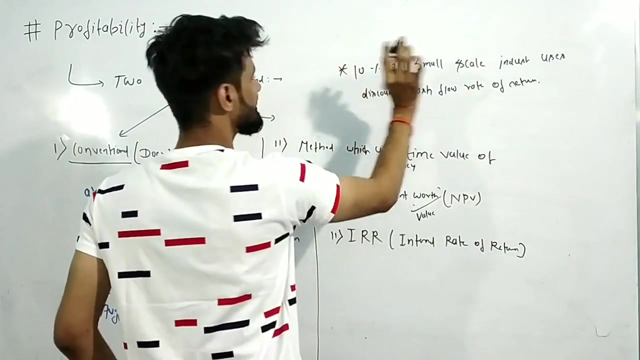 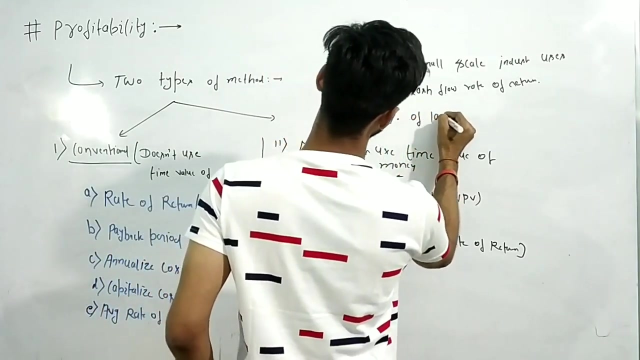 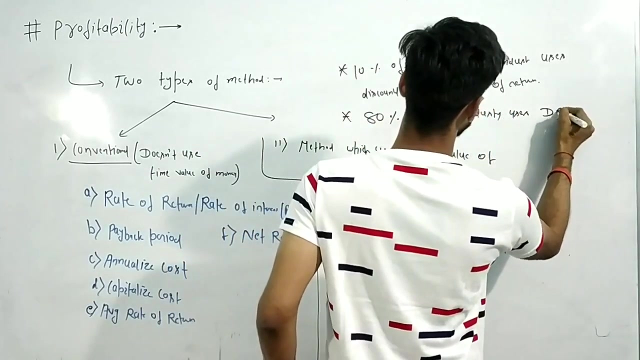 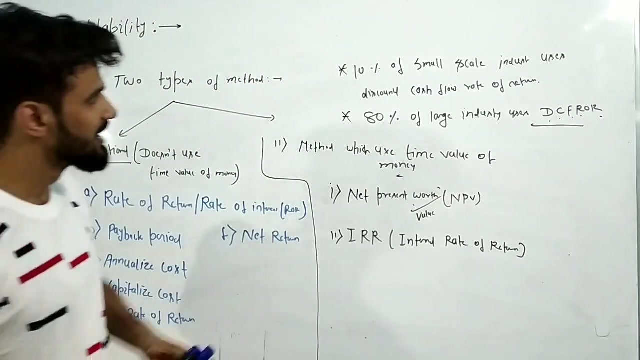 a small scale industry uses discounted cash flow rate of return. 10% of a small industry uses discounted cash flow rate of return And here you will see, 80% of large industry uses discounted cash flow rate of return, Discounted cash flow rate of return. Okay, So understand why. Because it's a analysis. 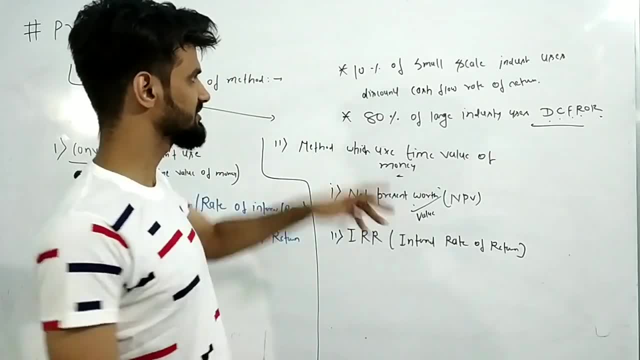 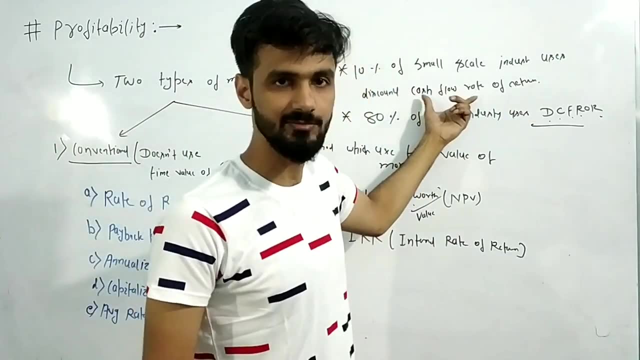 economics has analyzed the different different data for various industries. So he has found that 10% of a small industry is going to use the discounted cash flow rate of return. It is also comes in profitability analysis And 80% of the large industry uses discounted. 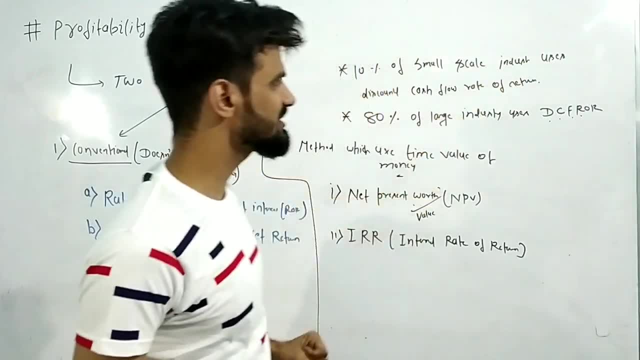 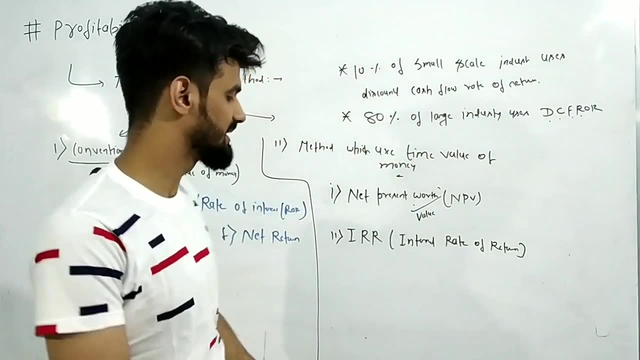 cash flow rate of return. Okay, So that depends upon the size of the industry. Okay, Because here you can say small scale industry, large scale industry uses discounted cash flow rate of return. Okay, And we are going to deal with the help of profitability. Okay, So that. 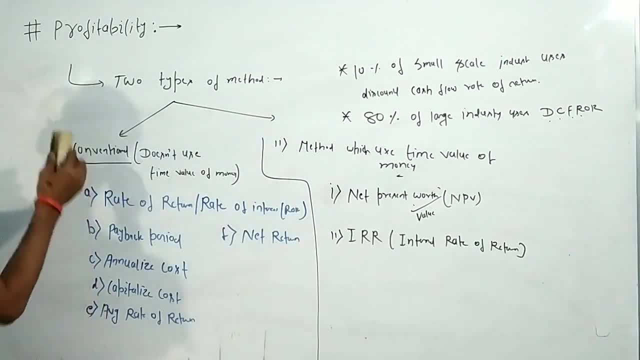 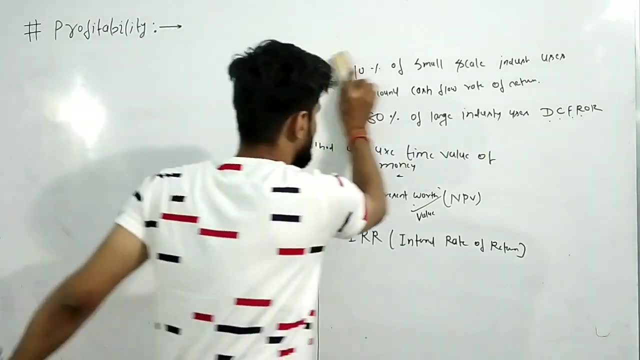 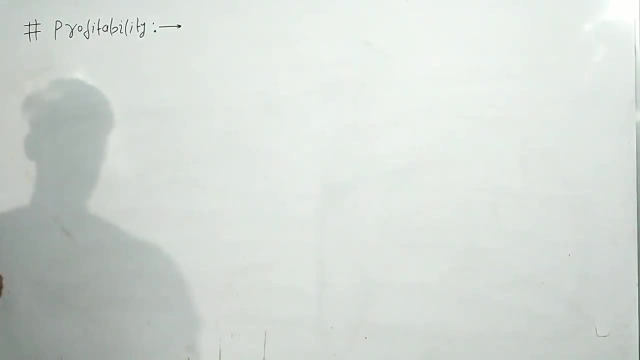 was the method that we are going to use in the profitability analysis. Now I am going to discuss each and every method categorically. First, we will start from rate of return. Okay, First I am going to start rate of return. Okay, First I am going to start rate of return. 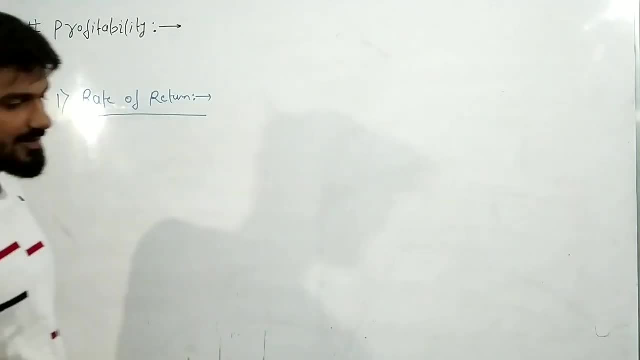 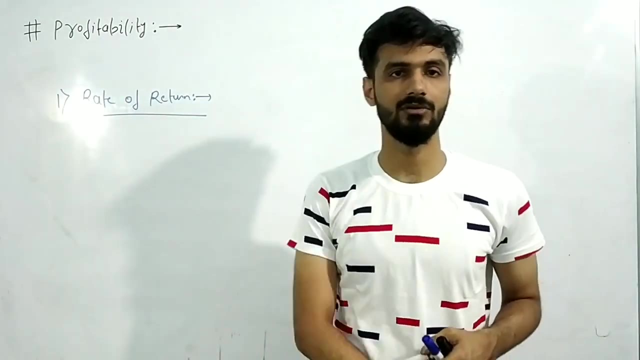 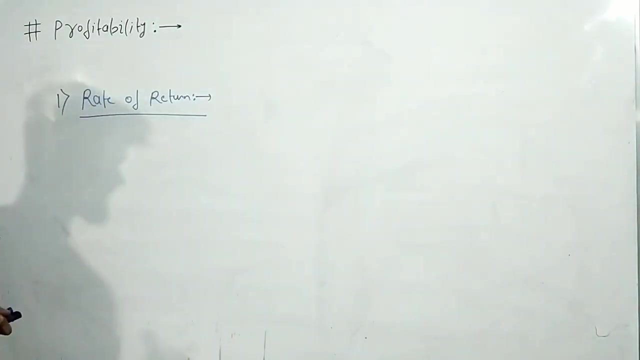 Okay, So many questions each and every year. If you will see the previous year questions of GATE examination, then 3 to 4 questions. that has been asked up to 2000 daily from rate of return, Okay, So it's very important topic. So first there are some assumptions, that is: 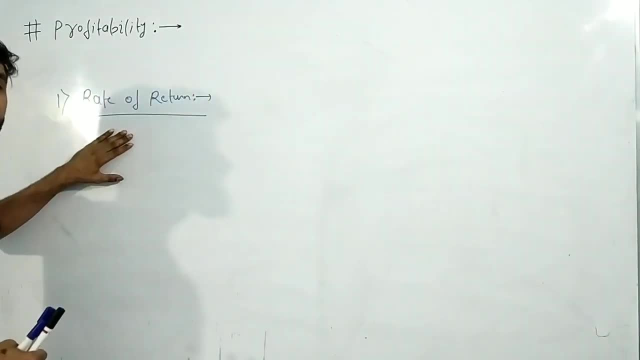 taken for the calculation of rate of return, for the profitability analysis. And I am writing the first assumption here. You can write it as assumption. Okay, So the first assumption is that it does not consider time value of money. So if you will see the first assumption, 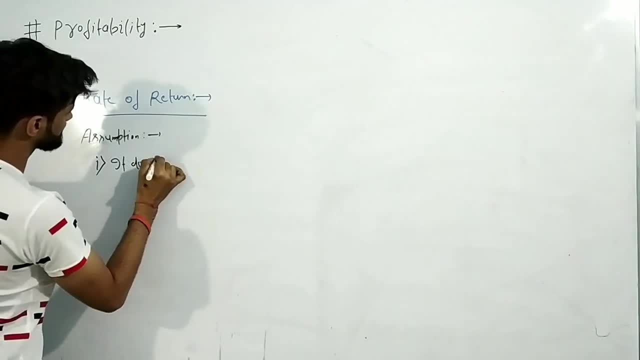 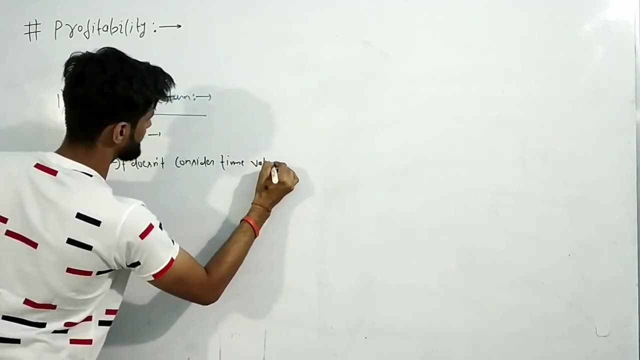 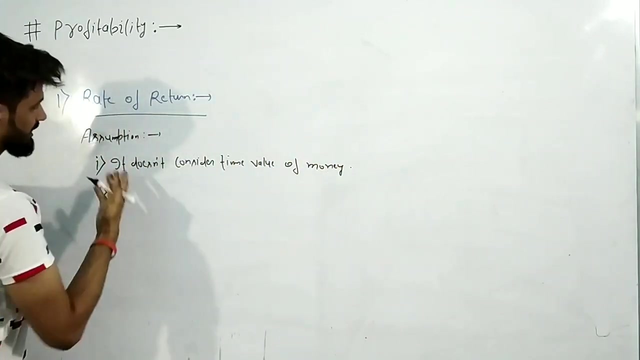 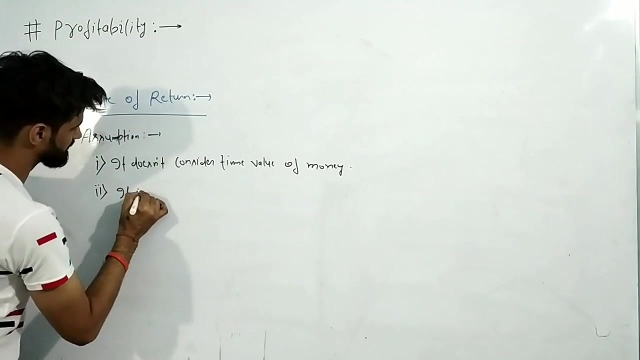 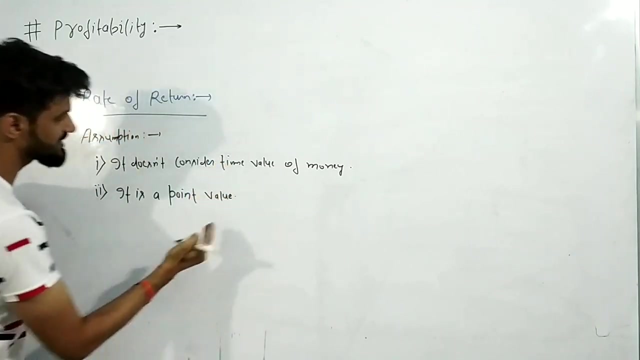 it does not consider time value of money. If you will see the second assumption then you can understand. it does not consider the time value of money for second only reason. Okay, It is a point value. My dear student, I am just teaching you in a very systematic way. 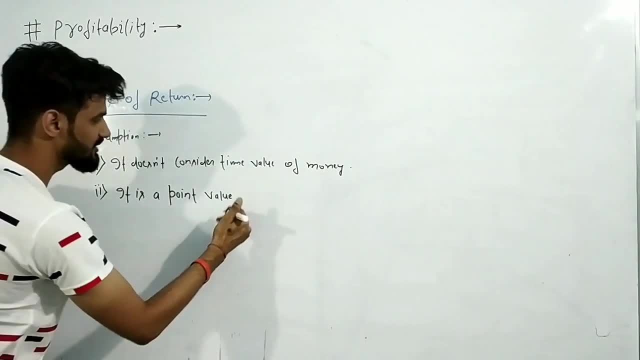 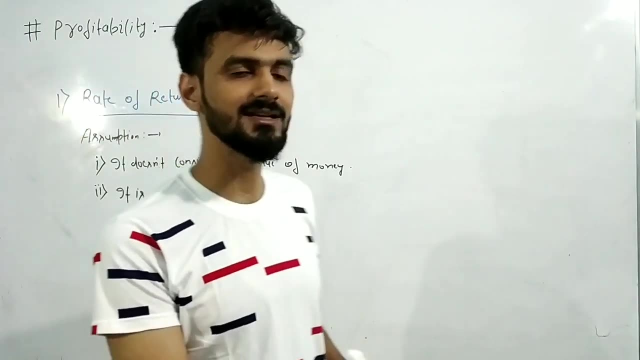 Change every topic I have there and I am writing in this so that you can remember it very easily, Because sometimes if you will see in the part examination or another examination, except from the gate, a small one marks question that can be asked from the definition or assumptions part. 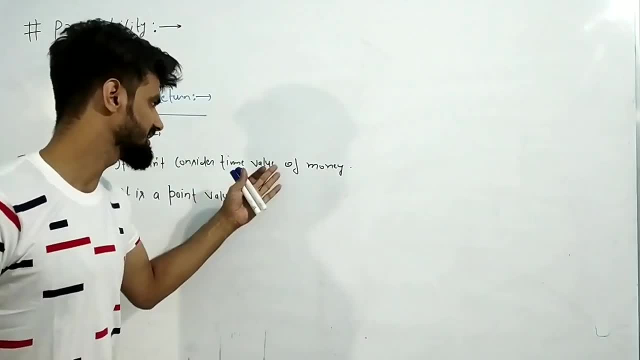 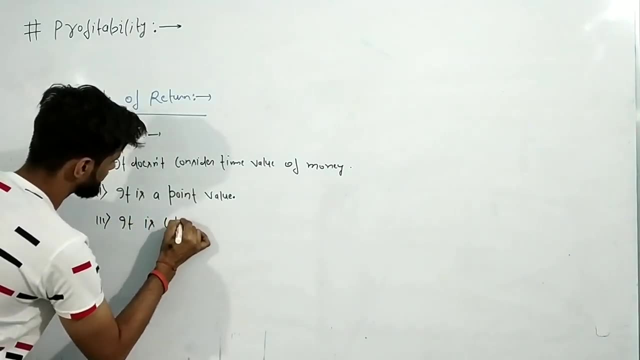 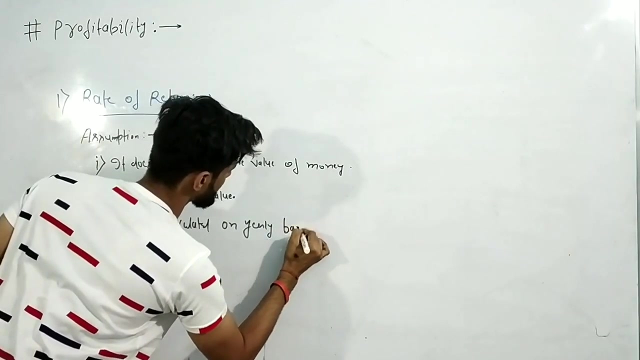 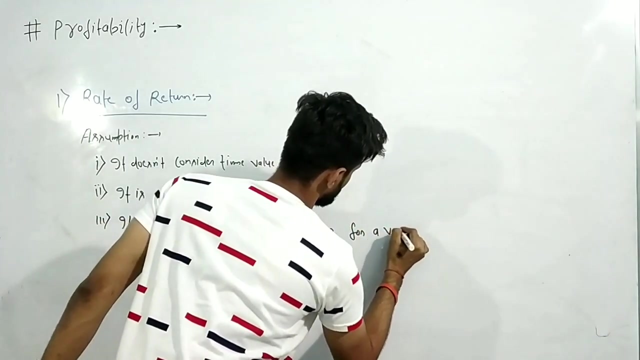 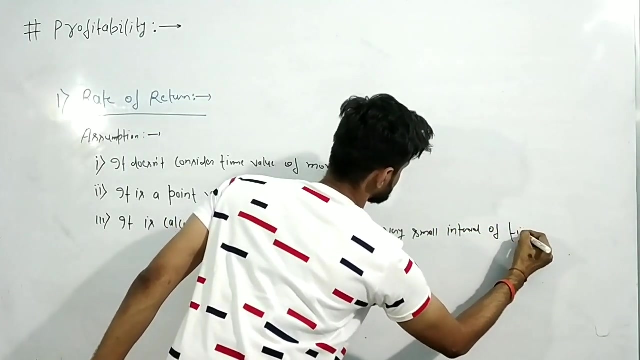 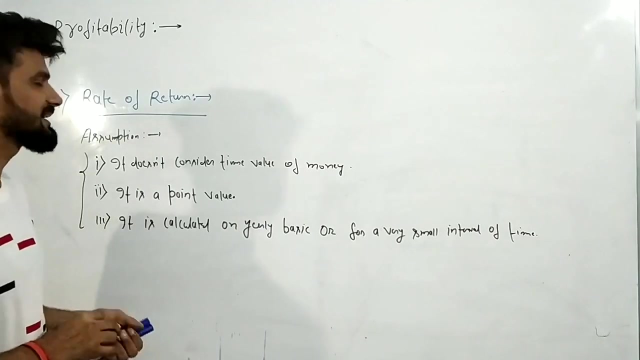 Or in interview they can be asked all these types of things. Third, it is calculated on yearly basis. or you can say that, or for a very small interview, Interview Level of time: Okay, Probably a small limit. So these three assumptions, that is taken, that has been taken by the economists for the calculation of rate of return. 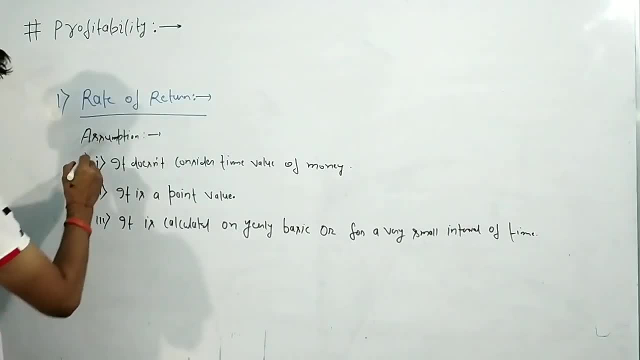 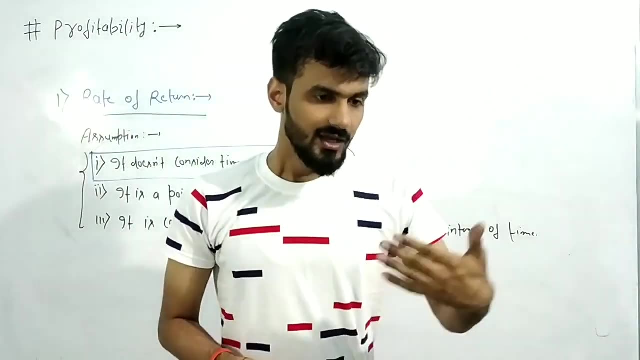 Understand one thing: It does not consider the time value of money. Already I have told you this is not going to consider. the time value of money Means the parameter that we will study in the time value of money. that is not going to consider in this method. 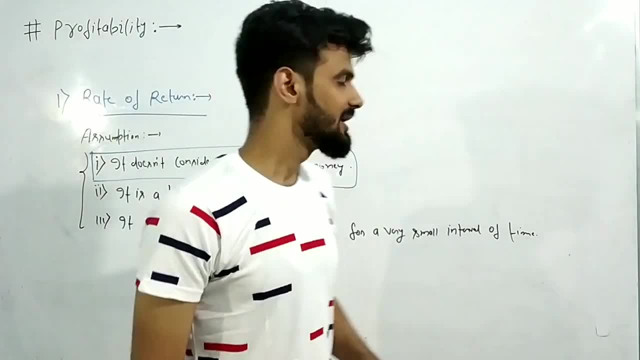 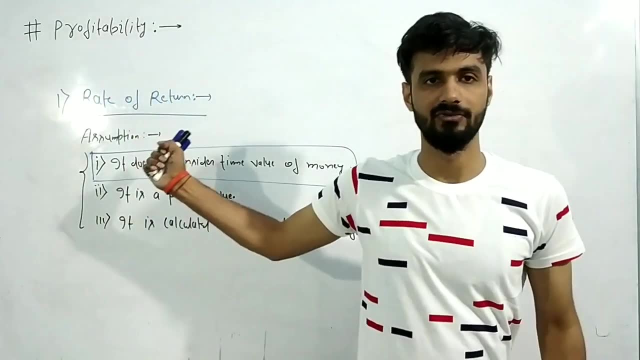 It is a point value. Why it is a point value? Understand one thing: If you are going to calculate the rate of return and telling you the formula of rate of return, then it is related to the profit. If you will see the rate of return, then rate of return is equals to profit upon investment. 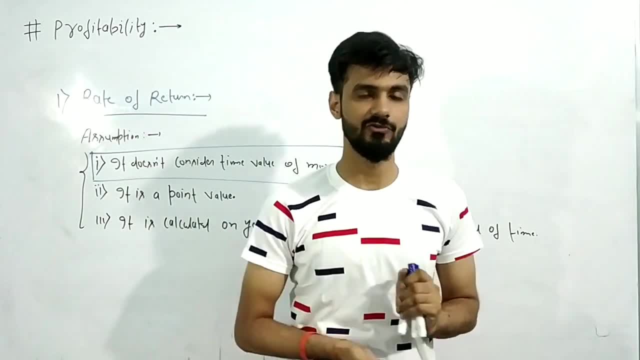 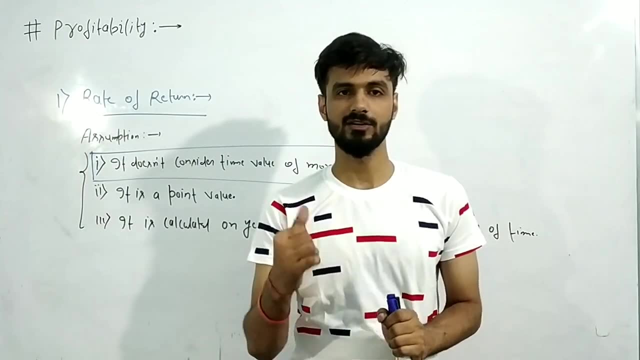 In a simple way. if you want to define the rate of return, then that is profit upon total investment. Okay, That is the rate of return. Okay, Now that is the profit in the numerator term of the rate of return. Okay, If you will see, each and every year, profit is going to be shared. 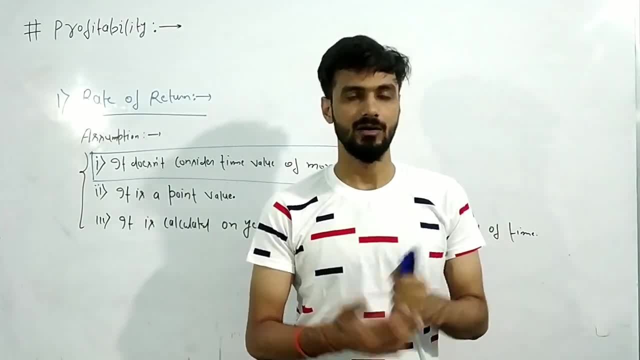 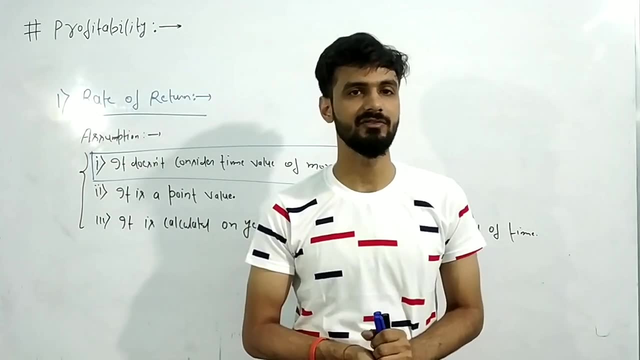 That profit depends upon the inflation and deflation of the material Of the country, Because the value of money is going to be changed from the particular inflation or deflation each and every year. So the profit is going to be changed each and every year for a plant. 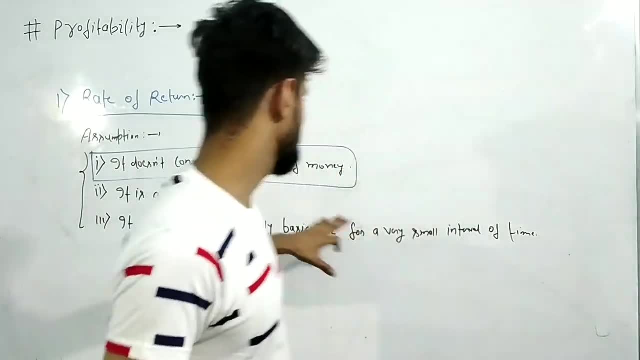 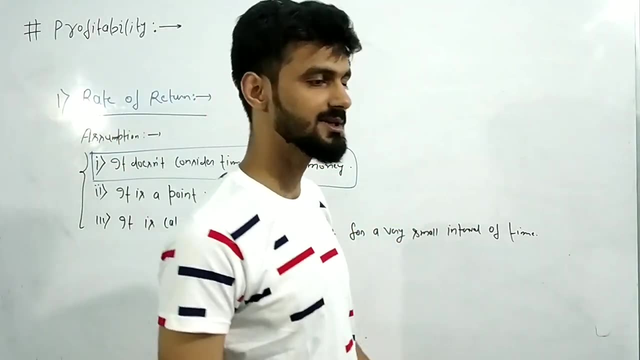 Okay. So if you will see here, then if profit is going to change, then what will happen? First year, you will get another rate of return. Second year, you will get some another rate of return. Third year, you will get another rate of return. 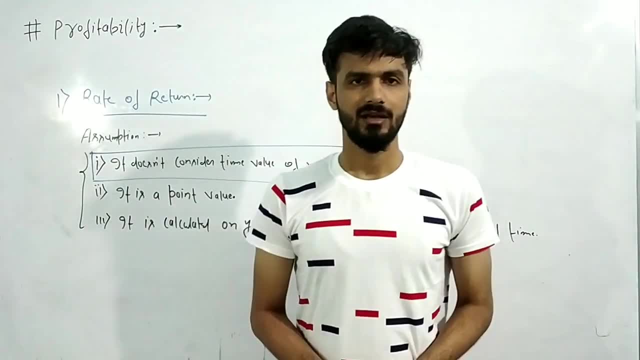 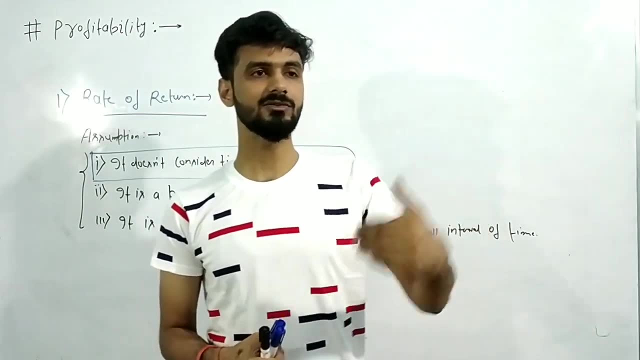 So it is very confusing thing. So you can't calculate the rate of return, So you can't calculate throughout the whole life period of the project for the rate of return. So it is better to calculate individually, for the individual year, each and every year. we used to focus about the rate of return. 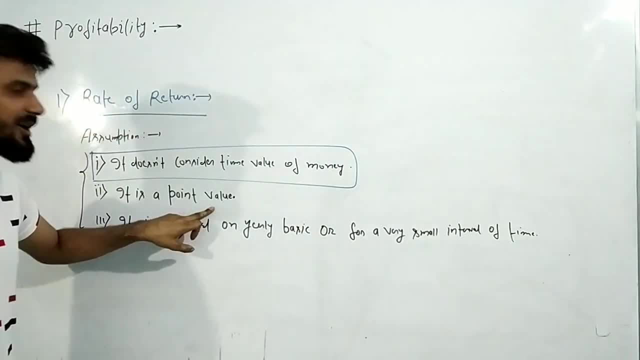 Okay, That is why we used to call it as the. it is a point value. Why? Because you can't calculate the rate of return throughout for the whole life period of the plant. Okay, Because that depends upon the profit. already I have told you. 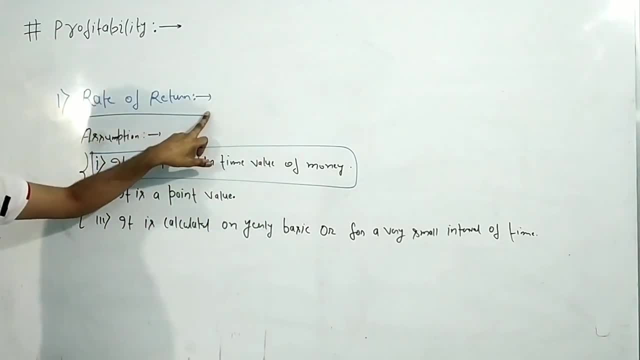 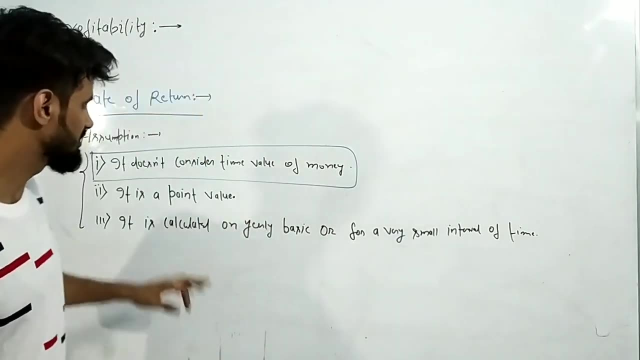 And if profit is going to be changed, then definitely rate of return will get changed. And how profit is going to be changed? Because each and every year, the value of money is going to be changed. Okay, Because it is a natural phenomenon, So due to deflation or inflation. 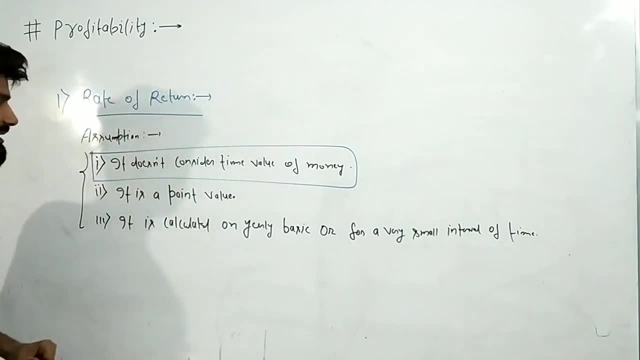 That is why the rate of return is going to be changed. So the economics is very. as a design engineer, we are very interested in calculating the value of rate of return for the yearly basis, Each and every year. Okay, And now if you will see the profit, then that depends upon the cash flow. 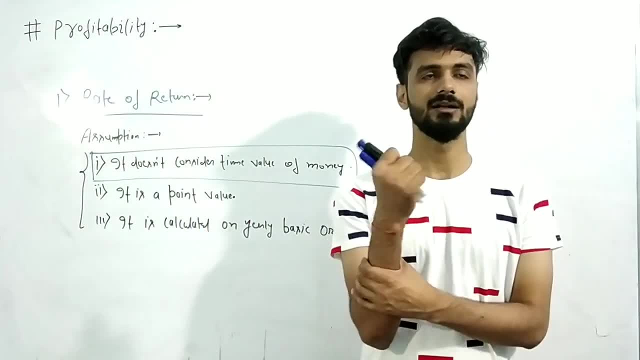 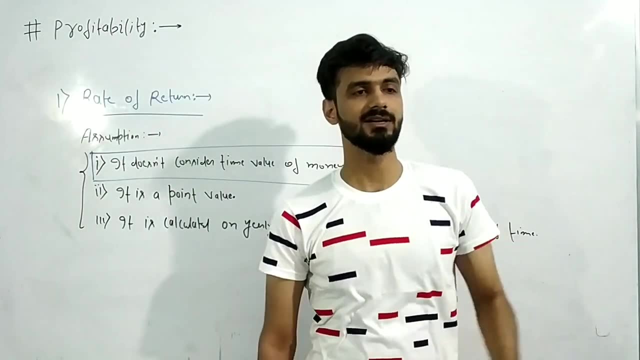 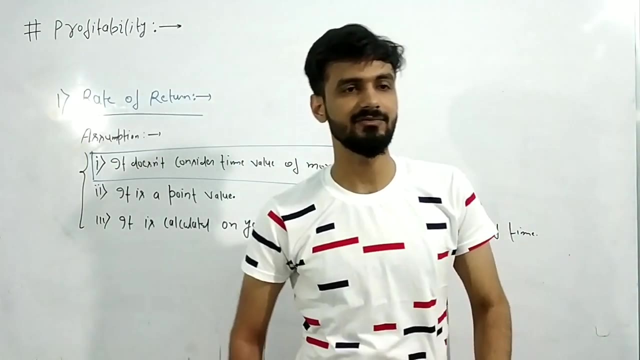 I will tell you the definition. in the definition, Where a term will come, that is, cash flow And that cash flow. or you can say the profit after tax. Okay, Profit after tax. So profit after tax depends upon the depreciation. Okay, And if you have studied the topic depreciation, there are various types of term that we have to study in the depreciation. 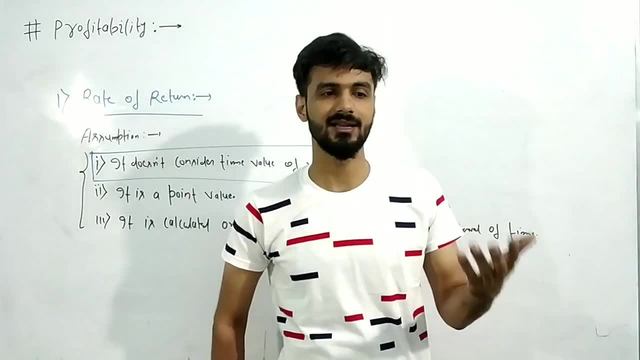 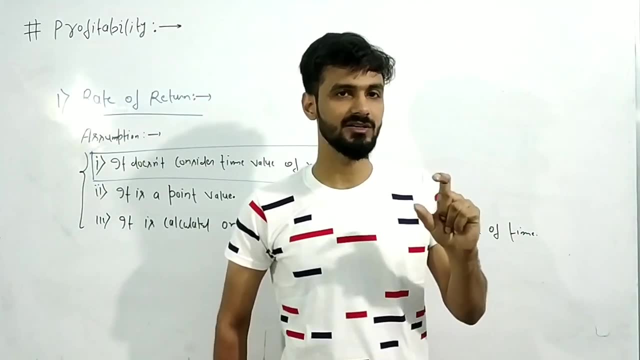 And first was straight line method, double decline method, decline method, sum of year, digital method, all these methods, But if you will see in the depreciation, only a straight line method used to give the depreciation value constant Each and every year. The depreciation calculated by a straight line method is constant. 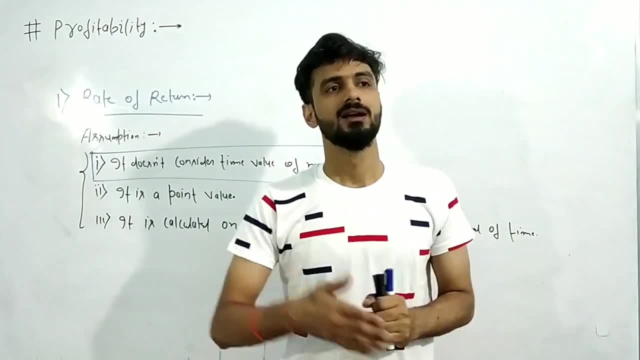 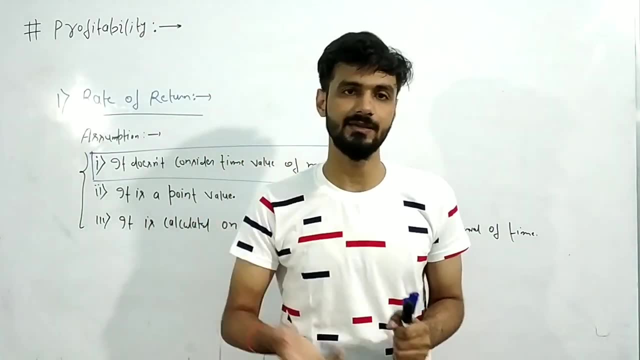 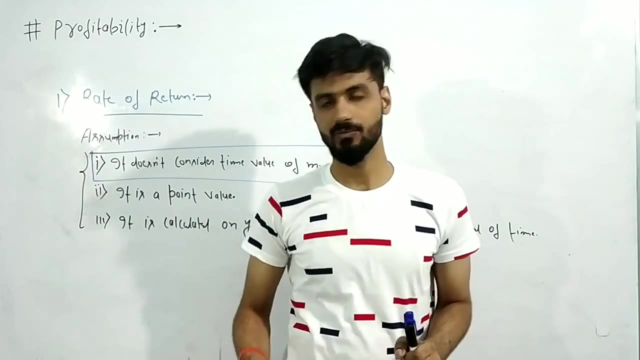 But if you are going to calculate a depreciation by sum of year, digital method, decline balance method or double decline balance method, then you are going to. you will see there is a different value of depreciation every year. Okay, So again it is going to change the profit and profit after tax, and again the rate of return will get changed. 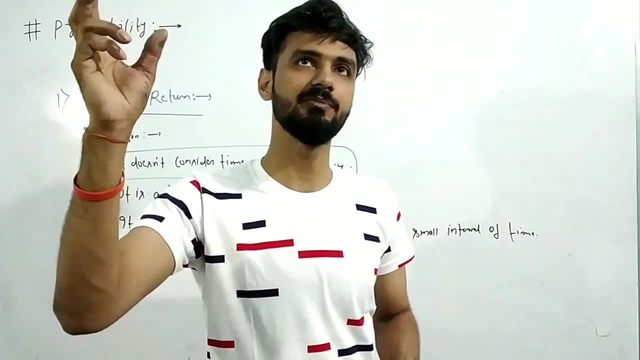 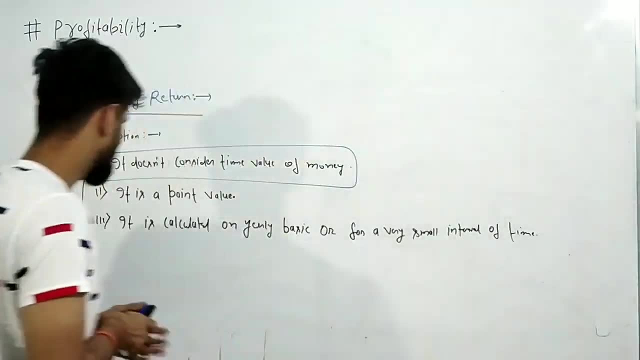 So it's better to calculate the rate of return for whole life period. We are- We people are- more interested in calculating the rate of return for a particular year. That's why it is called as a point value. That's why I have written here: it is called as a point value. 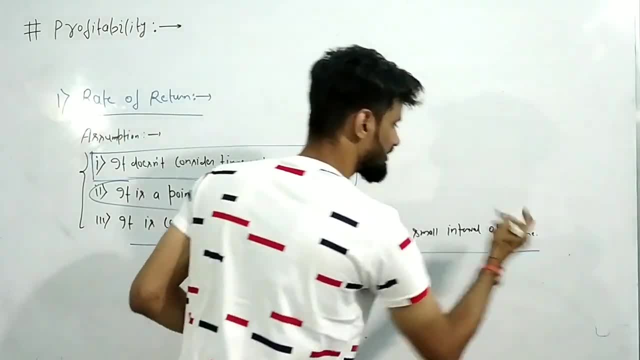 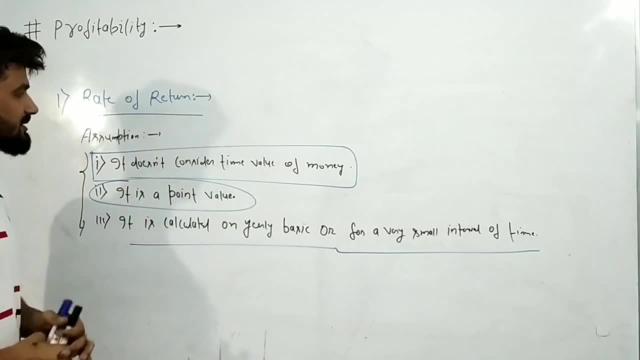 It is calculated only yearly basis, for a very small interval of time. Already I have explained it, Okay, So these three were the major assumptions in this topic. Okay, Now I am going to derive the derivation or formula for the rate of return, and how will we proceed about the question. 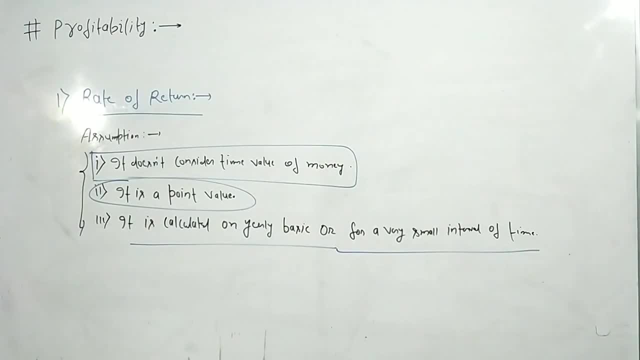 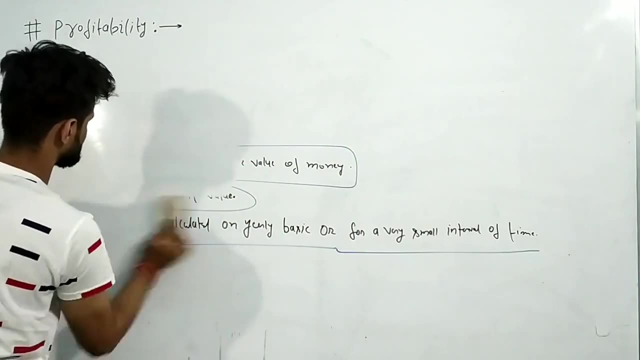 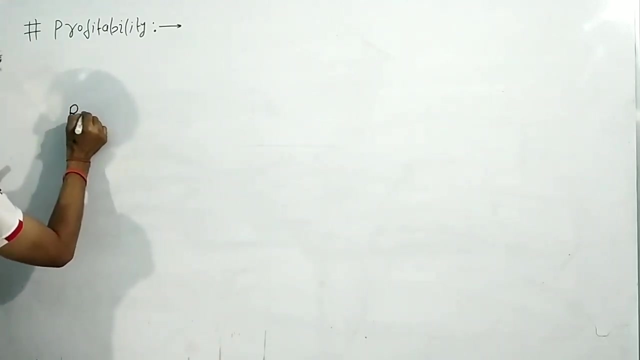 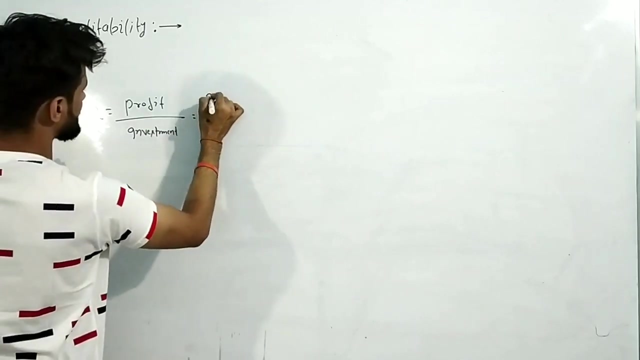 Okay, Okay, Okay. So you will see the formula of rate of return. The rate of return, simply, I am defining it in this way- Profit upon investment. Or you can define it in the profit before tax. Profit before tax upon FCI equals to profit. 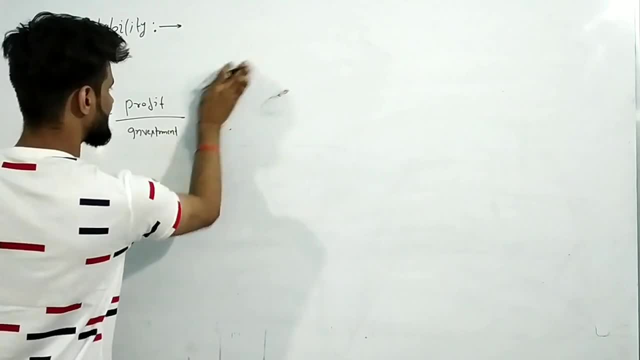 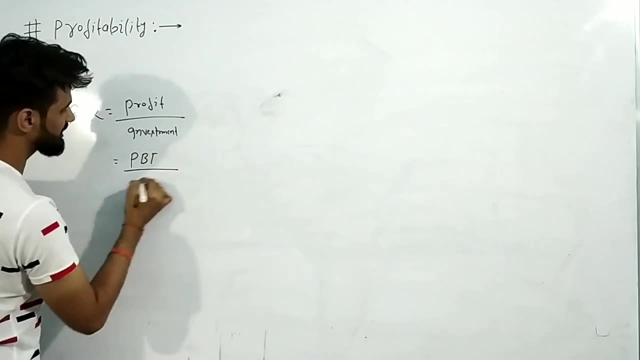 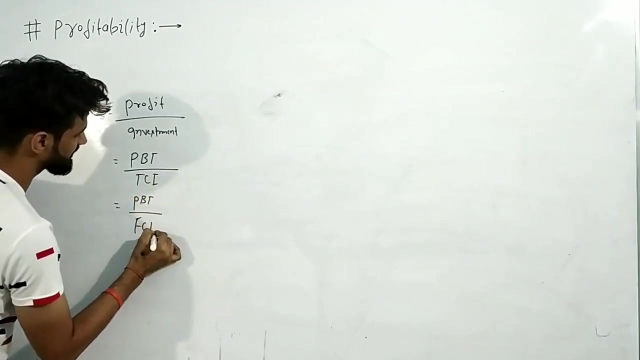 You can't write it. equals to form, Just there are different definitions. that depends upon your question, which is given in the question. I am writing it in this way: Profit before tax upon total capital investment. That is, equals to profit before tax upon fixed capital investment. 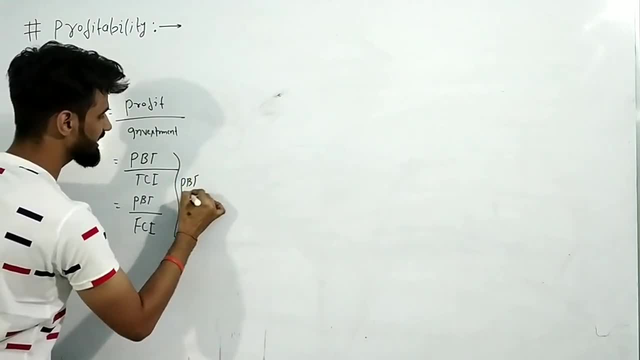 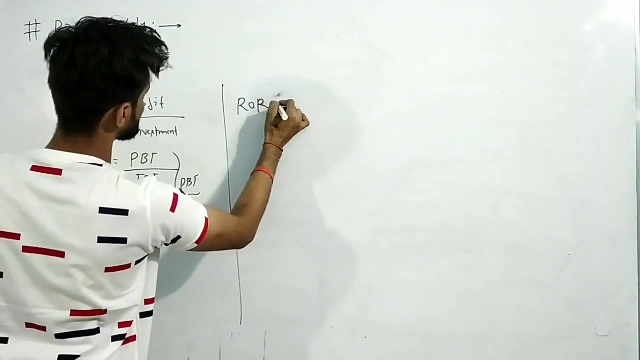 If profit before tax is given And FCI or TCI is given, Then you have to use this formula. Okay Now, if you will see, that is rate of return, That is, equals to profit after tax upon fixed capital investment. Or you can write it in there: 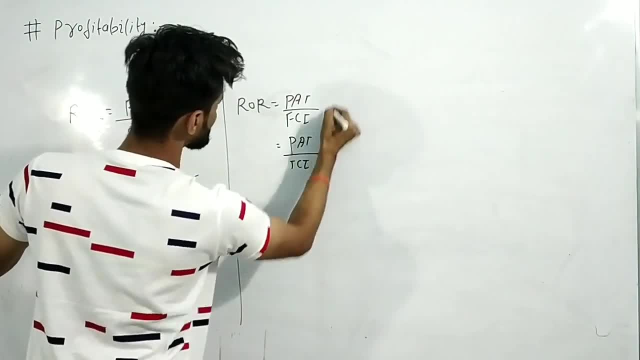 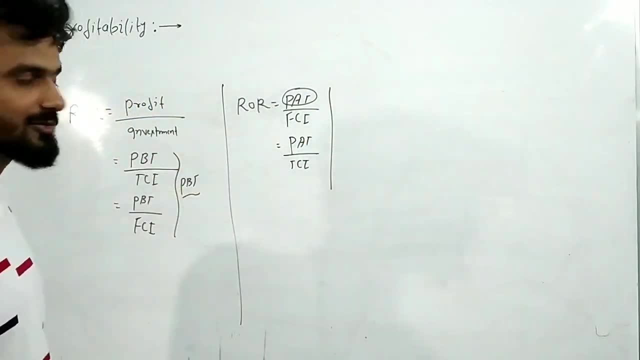 Profit after tax upon total capital investment. Okay, When we use this formula, When profit after tax is given, I will tell you how we will calculate the profit after tax. And if FCI is given and profit after tax you have calculated, Or there is flexibility in the question that you can calculate the profit after tax. 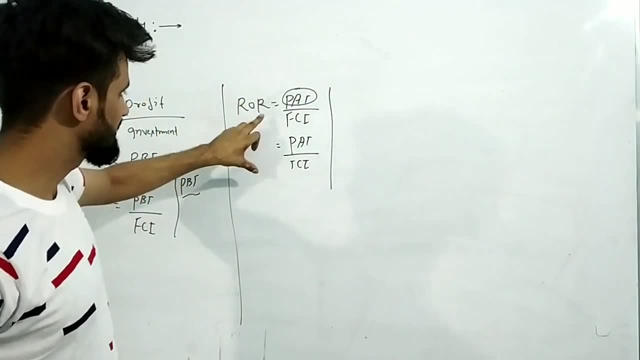 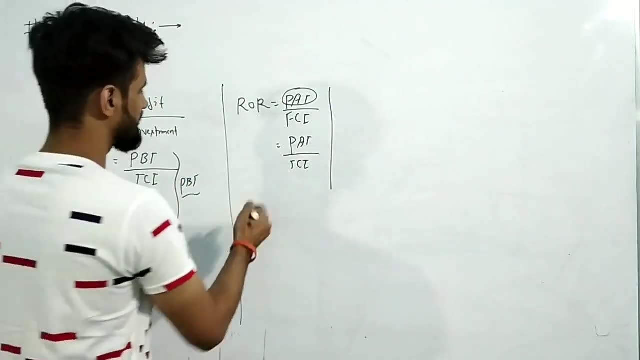 Then from there you can calculate rate of return from this formula as well. Now, if profit after tax you can calculate, Then TCI is given total capital investment, Then you can calculate this formula, Okay, From this formula. Now next formula for rate of return. 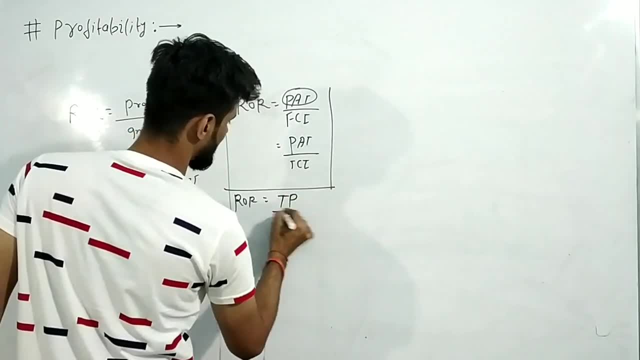 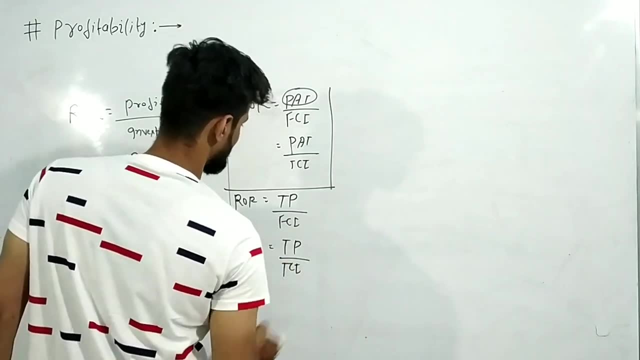 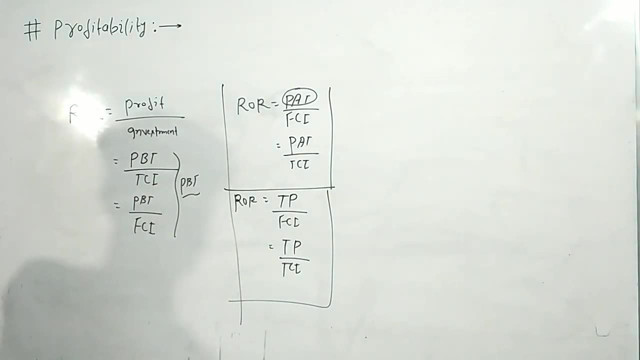 That can come from: taxable profit upon FCI. Anything can be written: Taxable profit upon TCI. Okay, These are the formula that we have to calculate in the profit rate of return. Okay, Now understand one thing: How will you calculate? 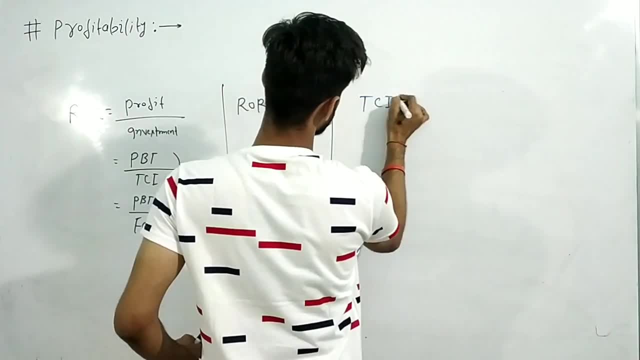 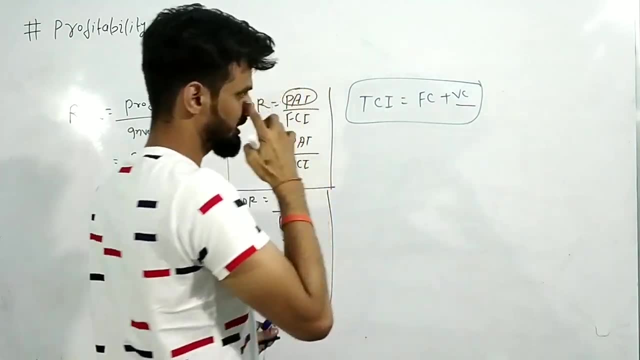 Just understand one thing: If you think about total capital investment, That is equals to fixed capital plus variable capital- Where will you use? If variable cost is also given Or fixed capital is also given, Then you have to use the formula of TCI. 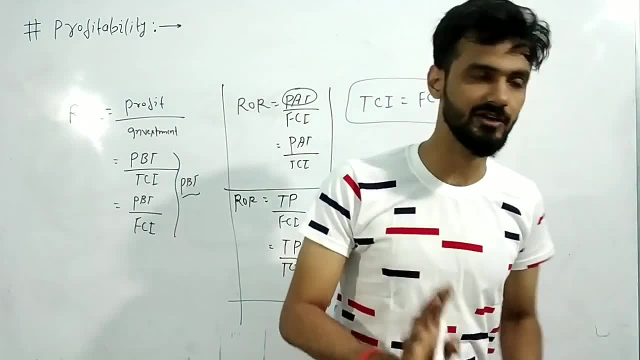 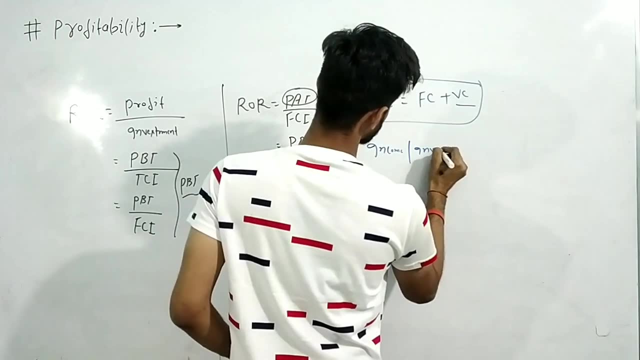 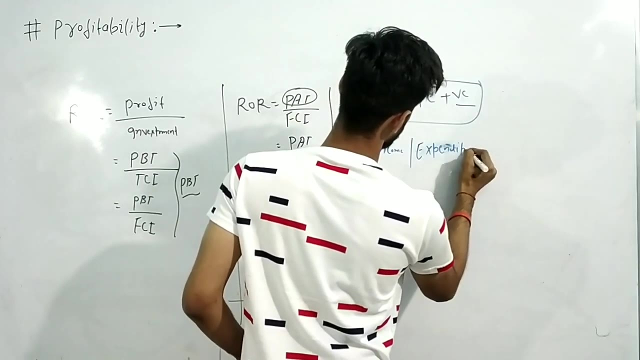 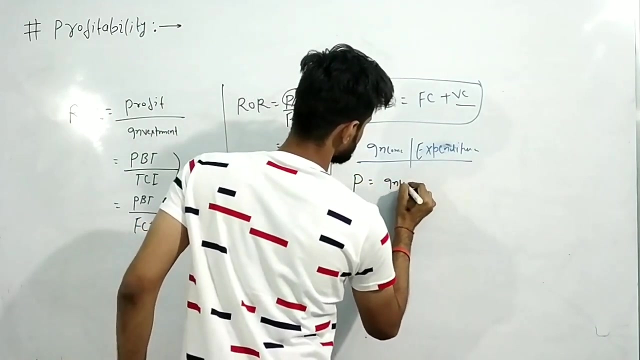 In that he is suggesting that use TCI. Okay, Now understand one thing: If only income is given and investment is given Or expenditure is given, If only these two terms is taken in the question, Then you will calculate: profit is equals to income minus expenditure. 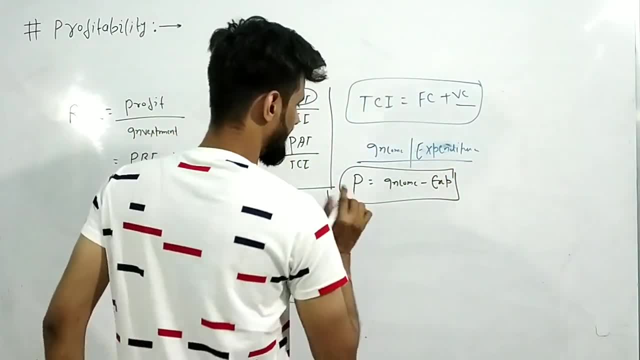 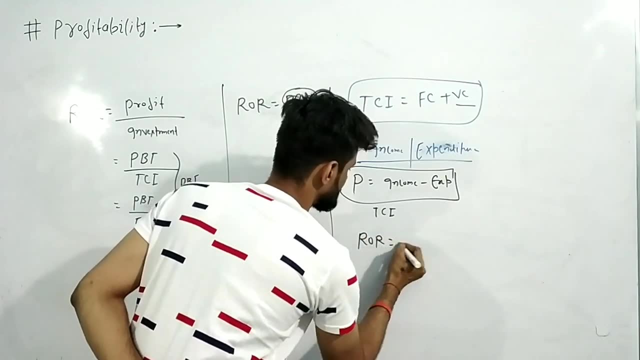 Income minus expenditure. Okay, From here you can calculate the profit. And if There is a flexibility for the calculation, If there is a flexibility for the calculation of total capital investment, Then you can calculate rate of return is equals to Profit upon total capital investment. 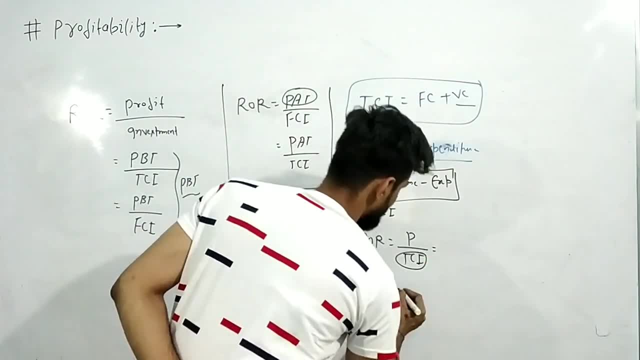 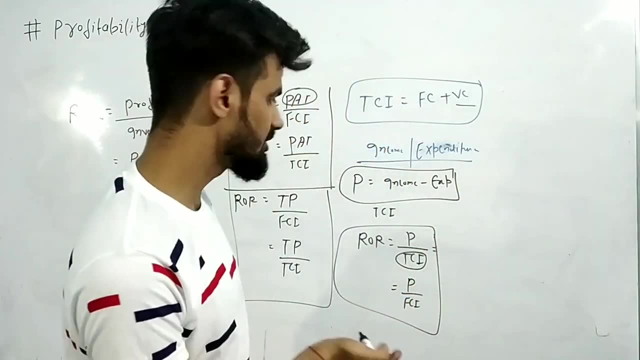 If total capital investment is not given, Then you can calculate that Profit upon fixed capital investment. Okay, Anything That depends upon your data of In your portion Which is given. Either only fixed capital is given, Then you have to divide the fixed capital. 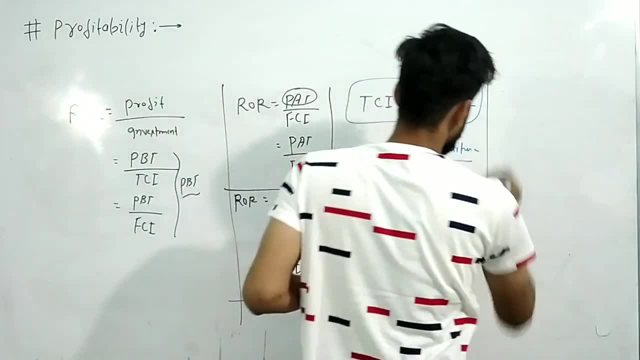 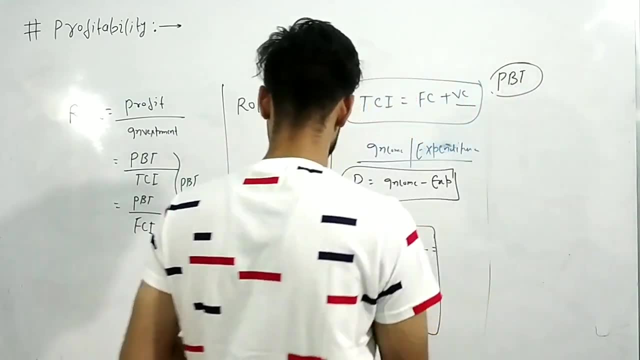 Then it will give the rate of return. Okay, Now understand one thing: Profit before tax. We are talking about profit before tax. Okay, How you can calculate Profit before tax. Now understand Generally if you use to calculate Profit before tax. 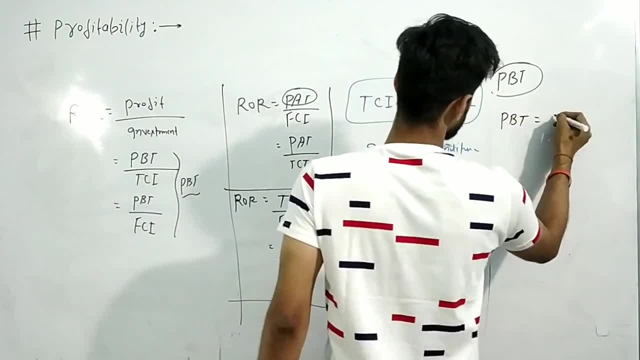 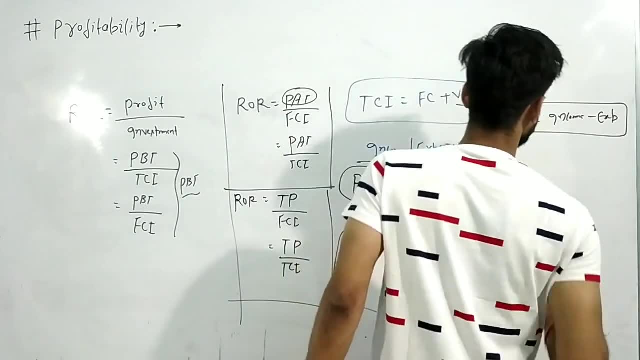 That is equals to Income minus Expendwehr, Income minus Expenditure. Okay, Now If you going to calculate to tax pay, Tax pay, Then you can calculate this in the way: Profit before tax. 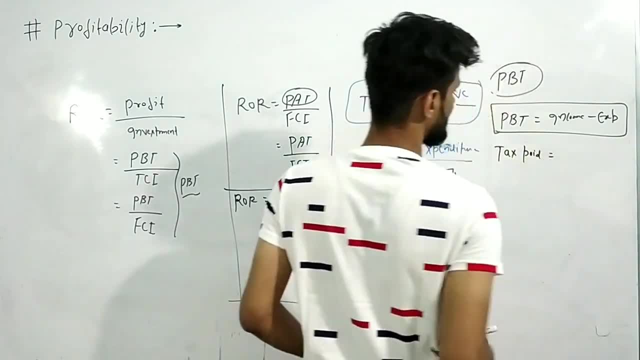 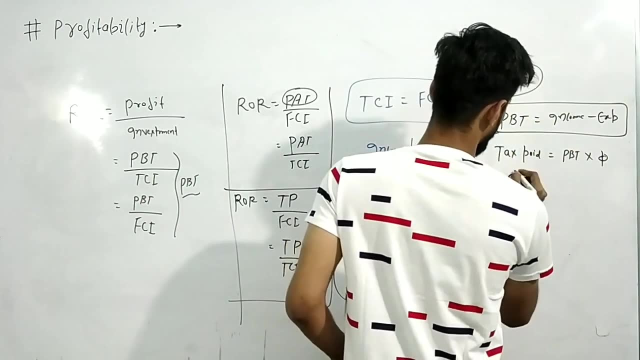 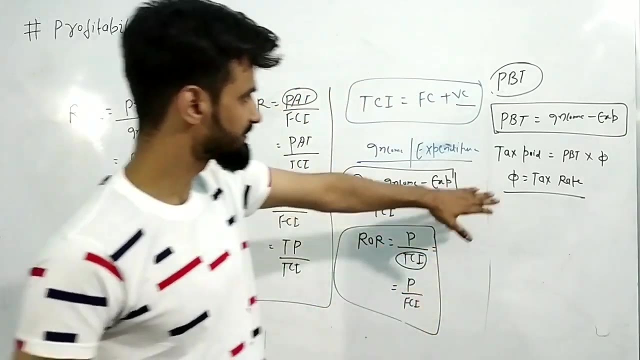 You are talking about income, much Expense. Now see here. Here you calculate income minus expense. Alright, Now, now too, Profit before tax multiplied by 5, And where 5 is tax rate, Where 5 is tax rate. Understand, this is the tax rate. 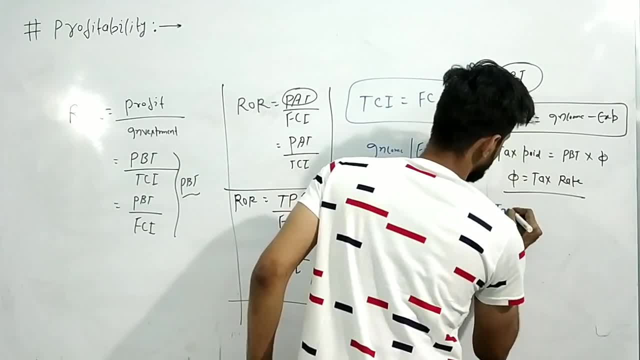 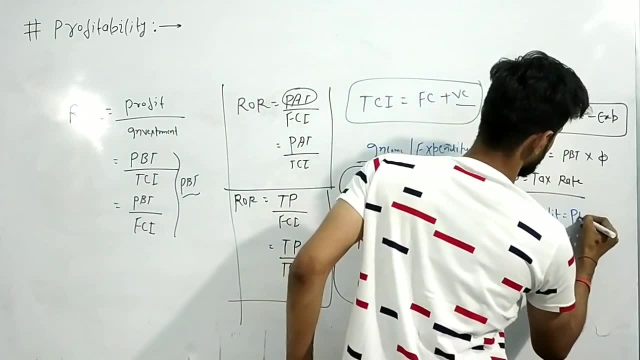 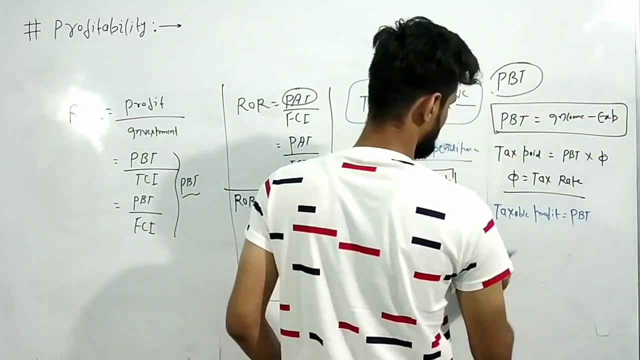 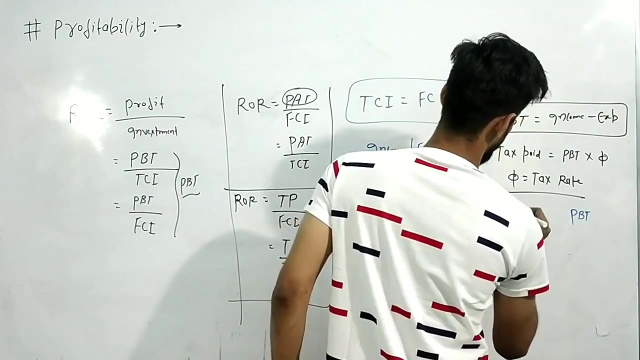 Now, if you want to calculate Taxable profit, So taxable profit is equals to. You are going to subtract profit before tax, Profit before tax. Just calculate the profit after tax, Profit after tax, Profit after tax. That is equals to PVT minus. If you want to calculate tax rate, 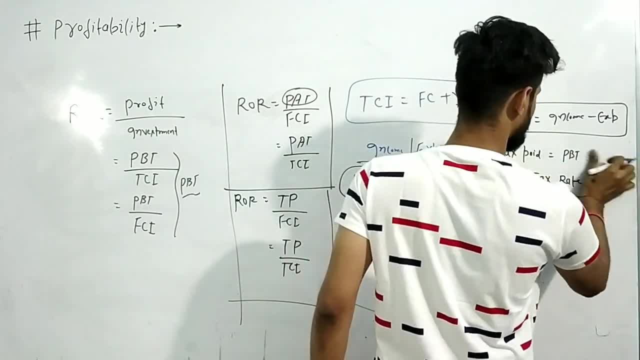 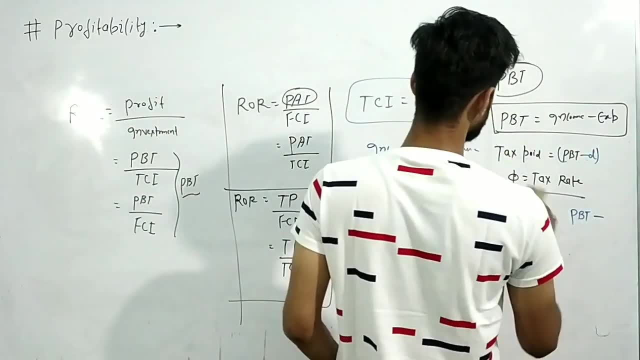 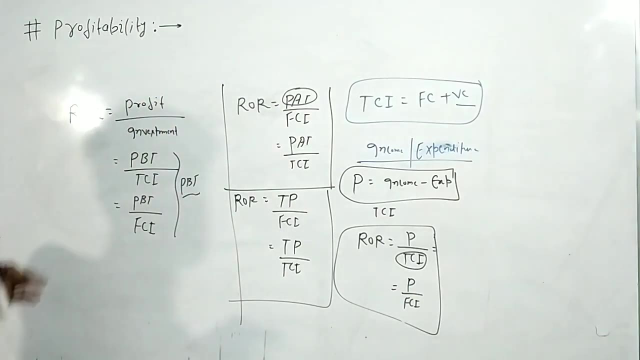 Then it will be equals to PVT minus depreciation, PVT minus depreciation. So this thing is Now. just understand one thing: How will you calculate profit after tax? How will you calculate this thing? So generally we have calculated PVT. Now I am writing here PVT, that is equals to: 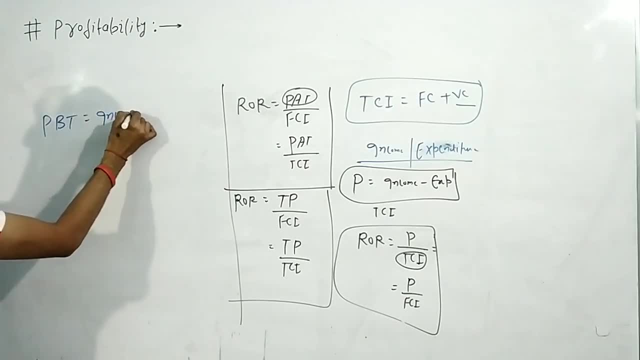 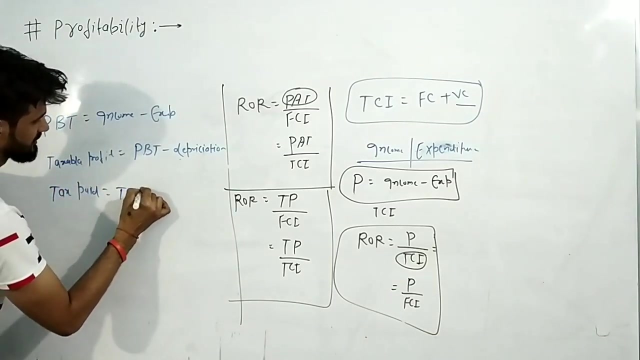 Income minus expenditure. Income minus expenditure. So if you want to calculate taxable profit, So if you want to calculate taxable profit, That is equals to PVT minus depreciation. I am writing: That is depreciation. Now, if you want to calculate tax pay, That is equals to Taxable profit. 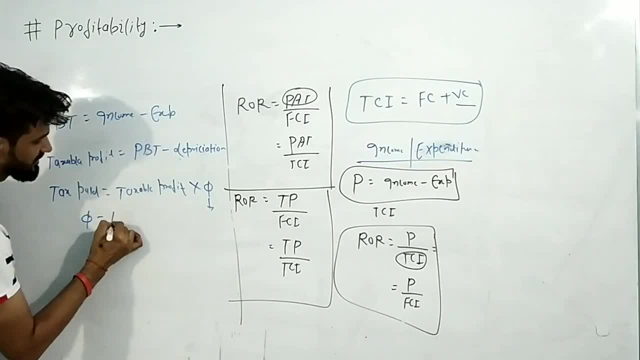 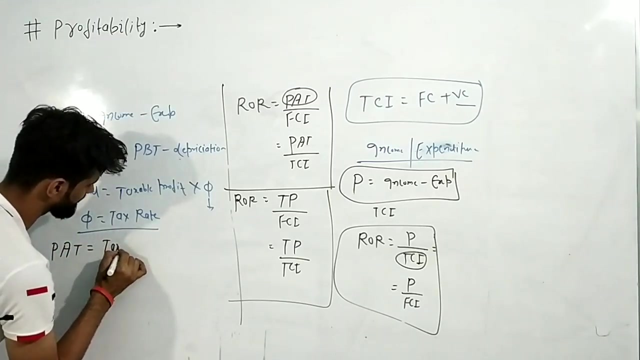 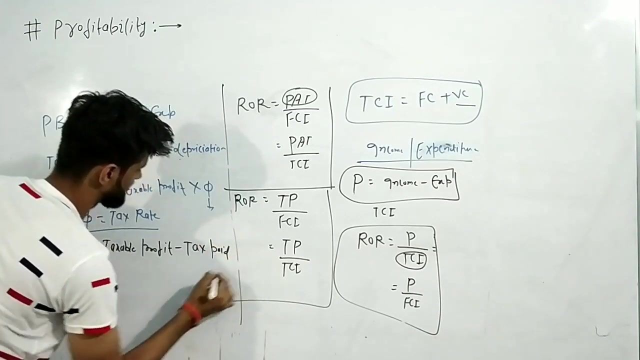 Might be calculated. 5 Where I am calculating, 5 equals to Tax rate. 5 equals to tax rate. Now, if you want to calculate profit after tax, Then you can calculate it as Taxable profit minus of tax pay. So you have calculated taxable profit. Taxable profit, that is, equals to: 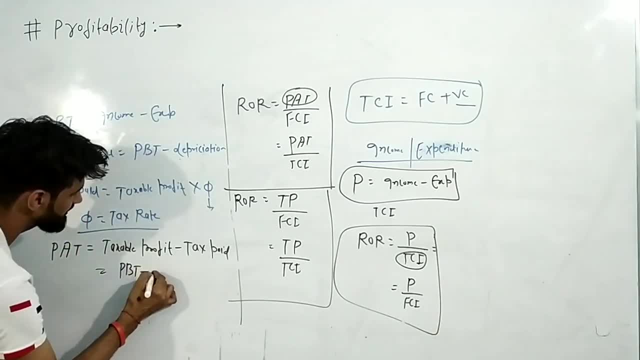 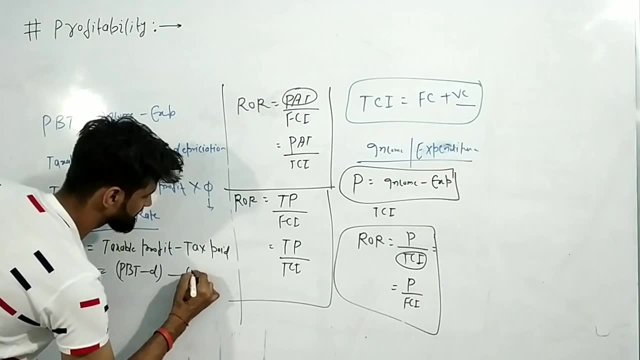 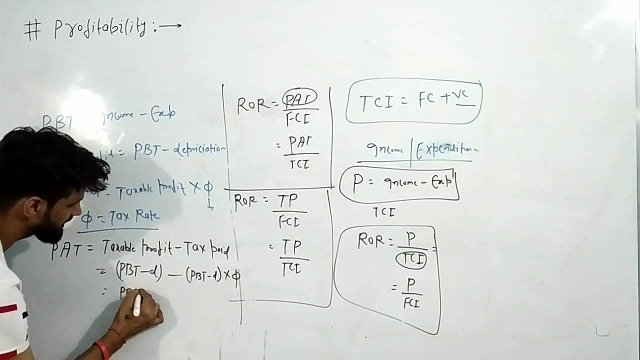 PVT minus depreciation. PVT minus depreciation minus tax pay. Tax pay is equals to taxable profit into 5. So you can write it as PVT minus depreciation into 5. So if you will calculate then it will be: You can get PVT minus depreciation Multiply with 1 minus 5. 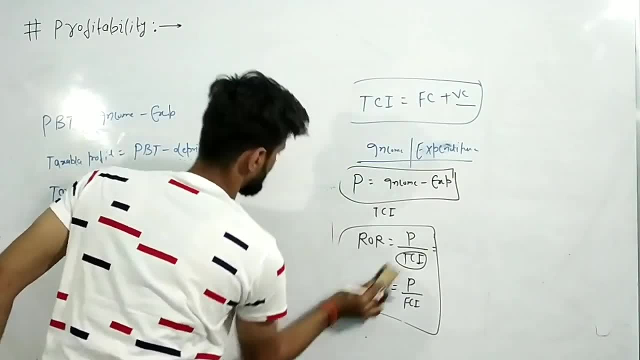 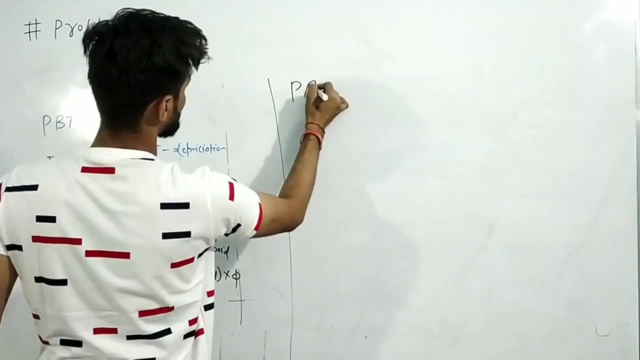 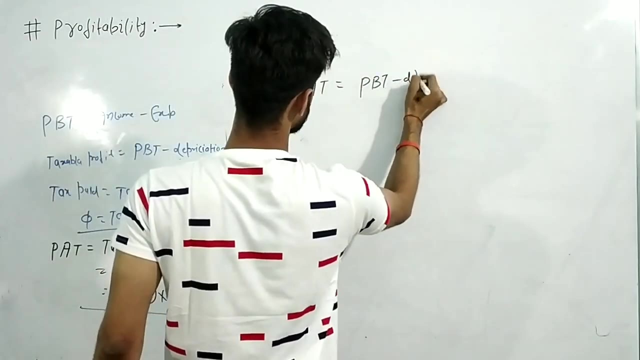 Okay. So if you want to write the definition Or formula of profit after tax, It is important you just understand one thing. So if you want to write profit after tax, So profit after tax is equals to Profit before tax, minus depreciation. Minus depreciation, PVT into 1 minus 5. 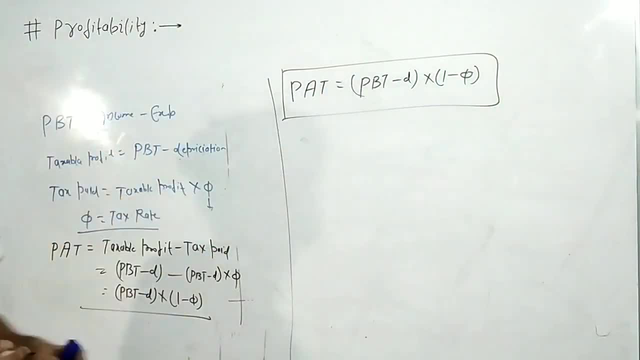 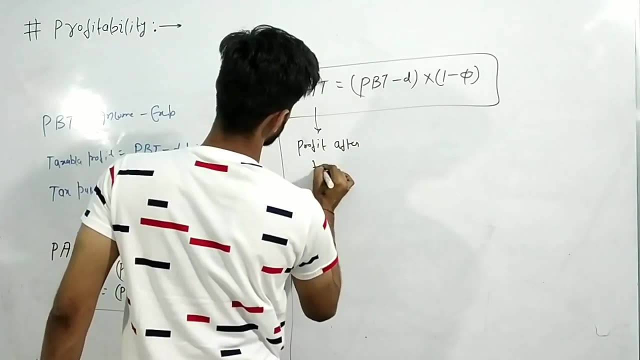 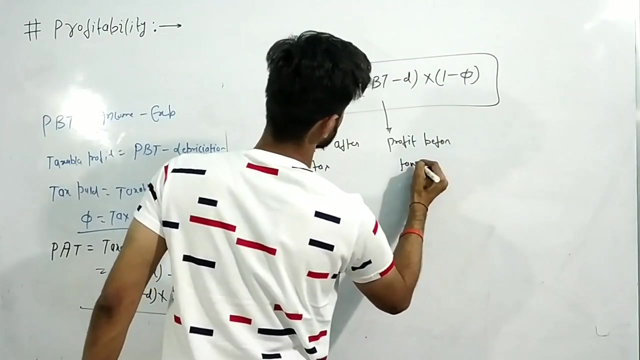 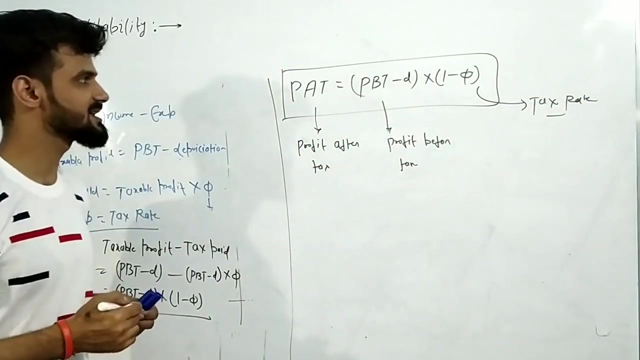 That is the formula of PVT. PVT: profit after tax. I am just writing here Profit after tax And here it is Profit before tax And here it will be tax rate. So it will be given in the question. Tax rate will be given in the question. Depreciation will be given in the question. 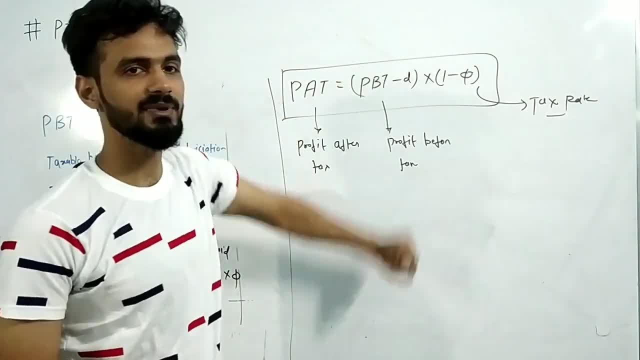 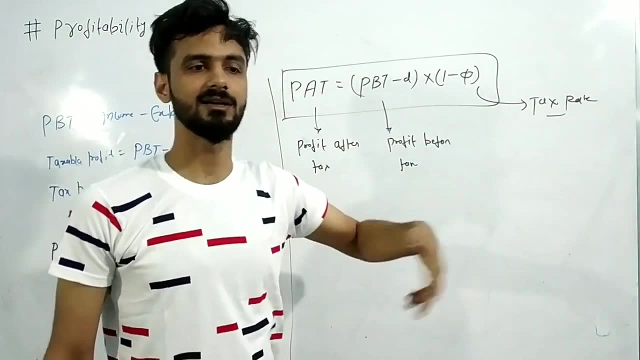 If depreciation is not given, then You can calculate the depreciation by Different kind method And if the question is providing you the flexibility of Calculation of depreciation by straight line method, Decline balance method, Double decline balance method or Some of your decision Depends upon the scenario. Which types of data is available in the question. 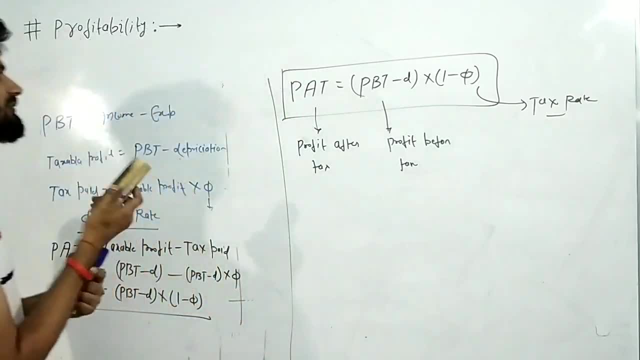 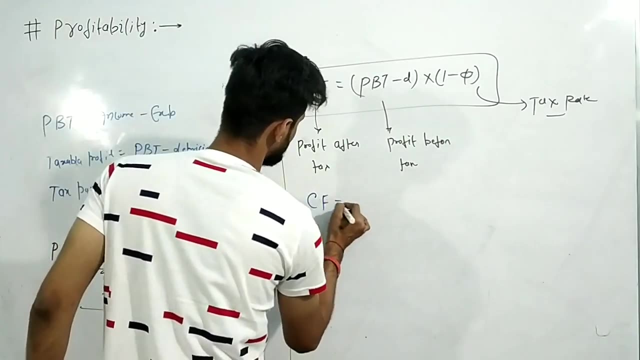 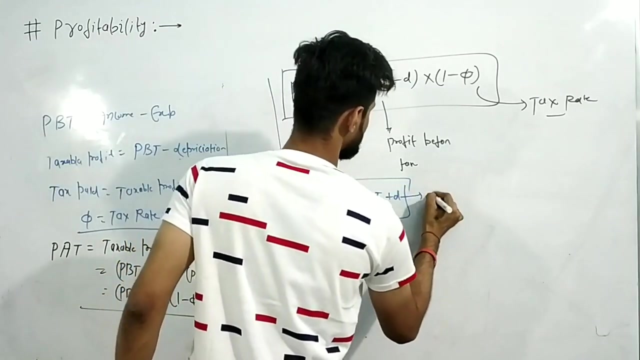 Okay, So I think, up to this, you can calculate the Profit after tax. Now One term that is more important here: How will we calculate the cash flow? Cash flow is Only Profit after tax plus depreciation. Here it is depreciation. So in this way you can calculate the profit cash flow. 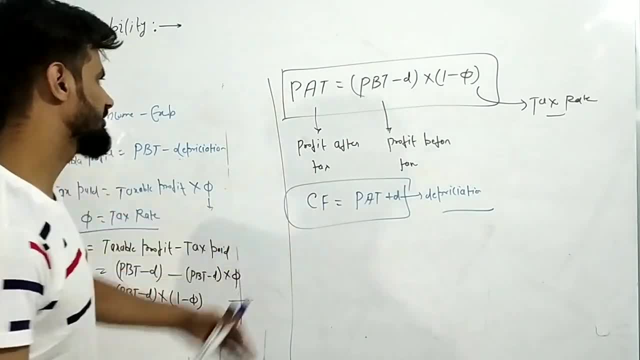 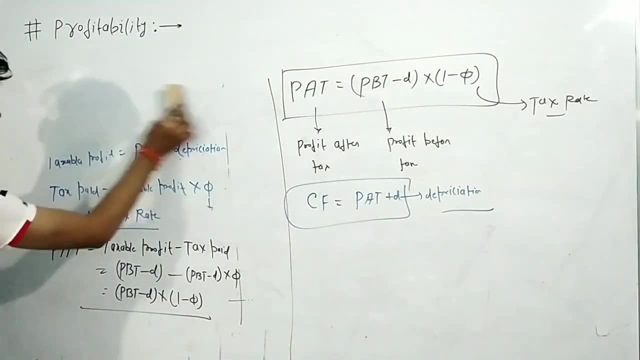 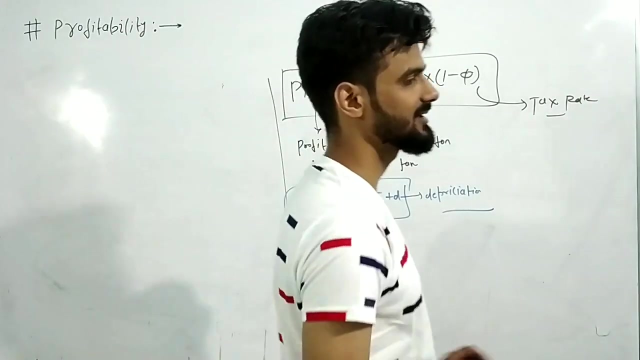 Okay, So this was the various formula That I have derived here For the calculation of rate of return. Now I am going to discuss about the cumulative rate of return. So I think, up to this point, it is very clear. now In the next lecture I will discuss about the cumulative rate of return. 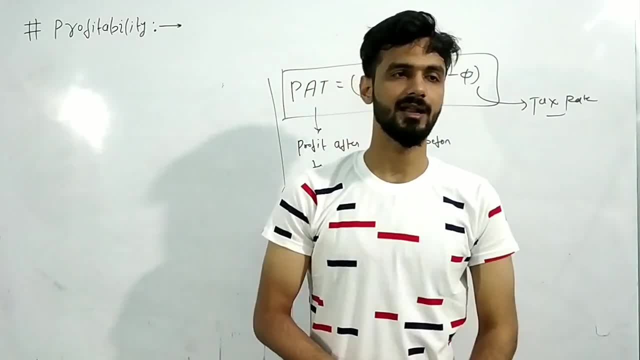 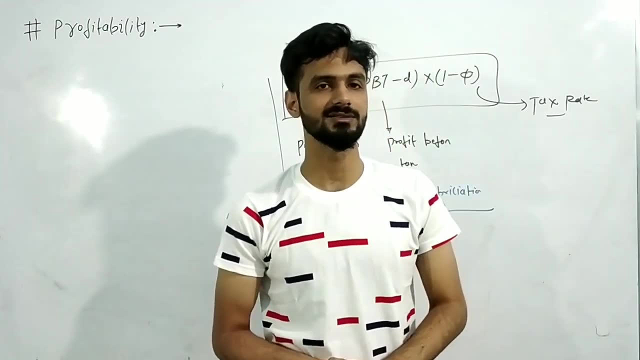 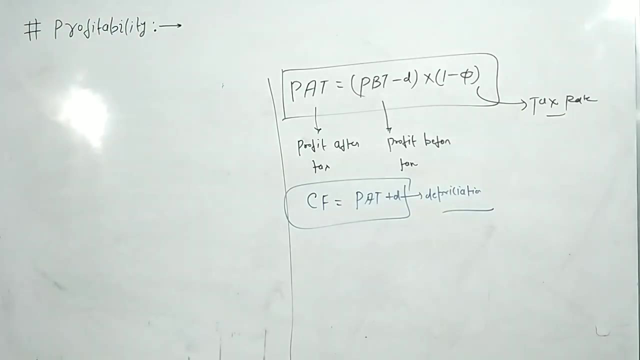